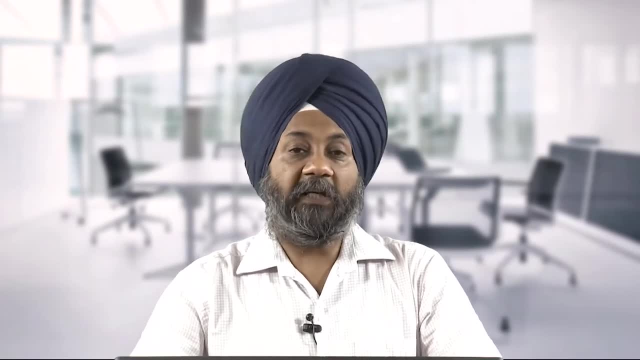 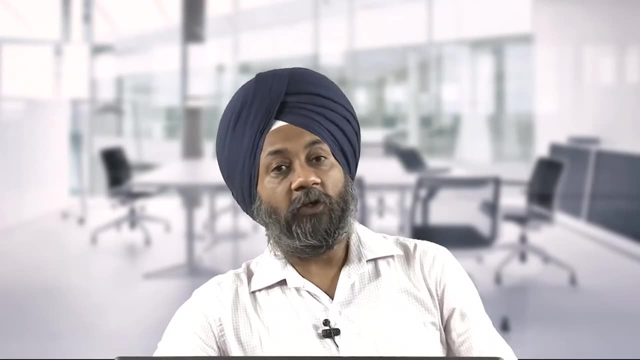 that you have understood or theories that you have studied related to the manufacturing processes. Normally in our curriculum we talk about the process. we talk about the kind of raw materials it can process. We talk about the process mechanism: how the material will be cutting, converted into the 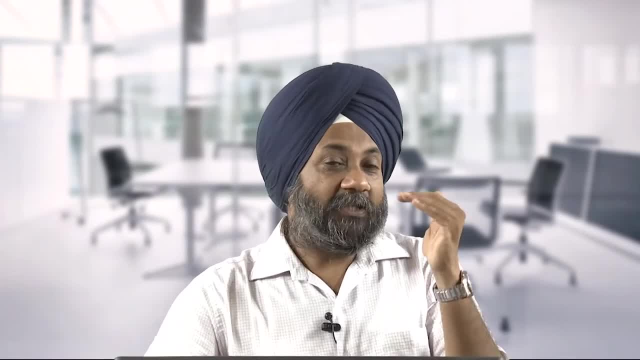 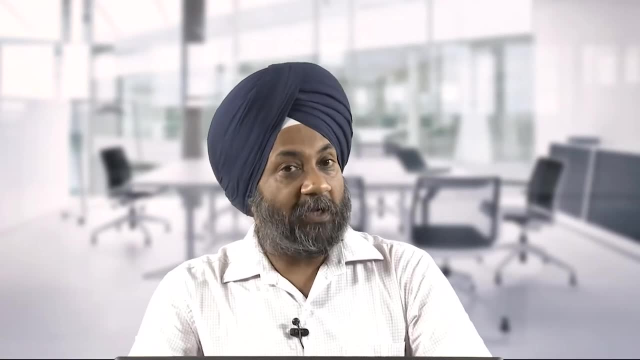 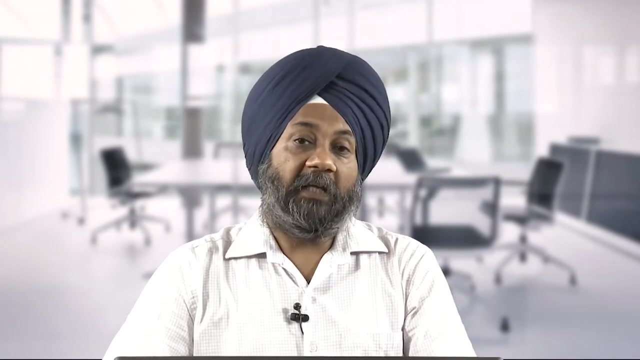 final product, But usually we lack a discussion regarding that. what are the product design guidelines related to that process? that if the product has to be made by a specific process, for example, say, metal die casting or pressure die casting, In that case what guidelines we must keep in mind when we are designing the product? 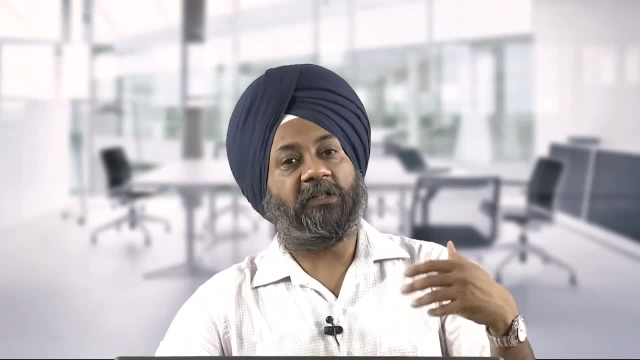 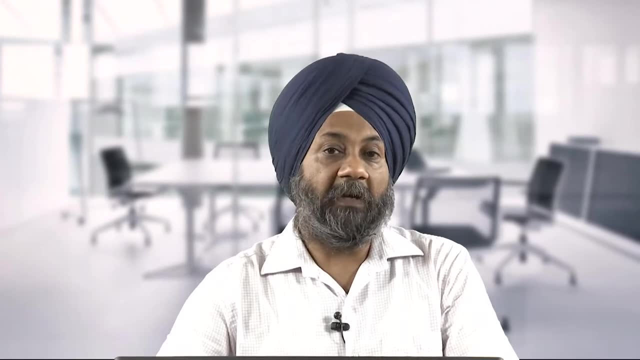 Usually pressure die casting is taught: The design of the die, the design of the ejector pins, the cooling system, the pushing mechanism for the metal, the heating mechanism for the metal. So all that is taught, but sometimes we have very little discussion about the products. 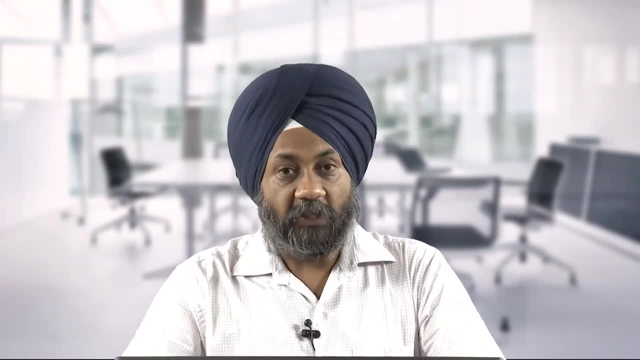 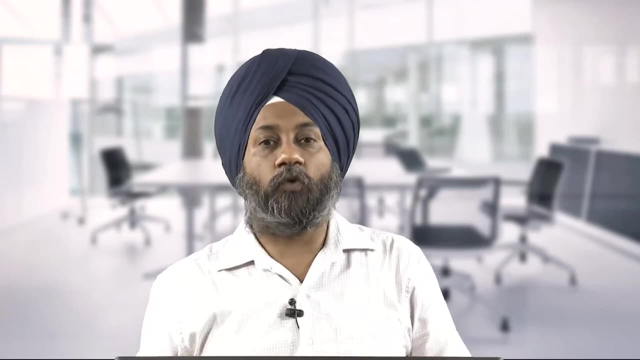 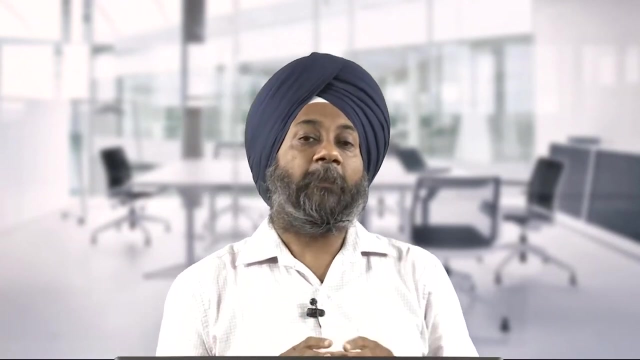 that should be made by the pressure die casting process. So this course, basically, is focused on these type of guidelines And it is a very, very condensed course of 20 hours and we have tried to include many possible processes That are used or that are maybe in that are employed for during the product development. 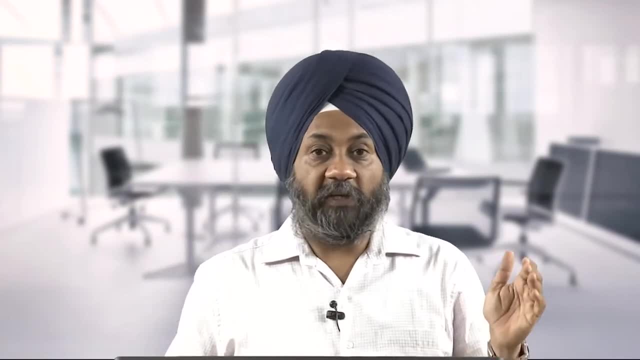 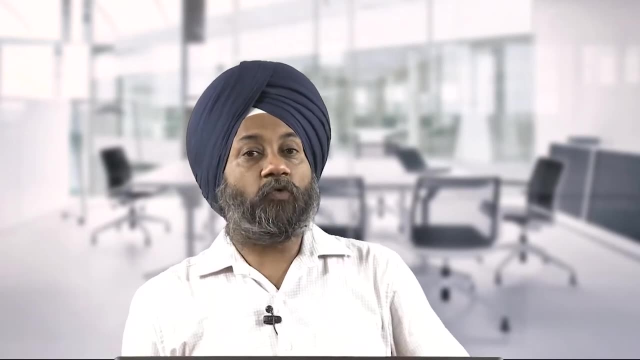 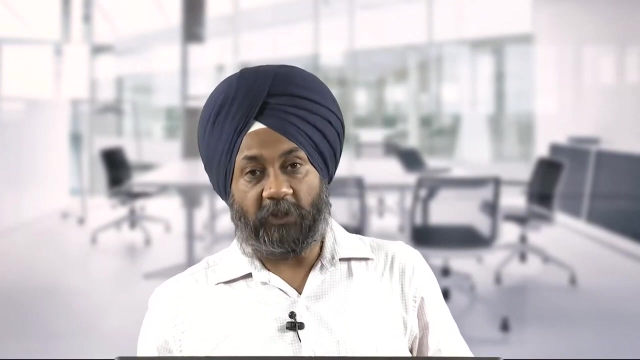 cycle. So, if you remember, in the last 5 weeks we have been discussing the various topics and we have then started the discussion related to the individual process, And the processes that we have already covered include sand casting, pressure, die casting, compression molding, extrusion, injection molding. 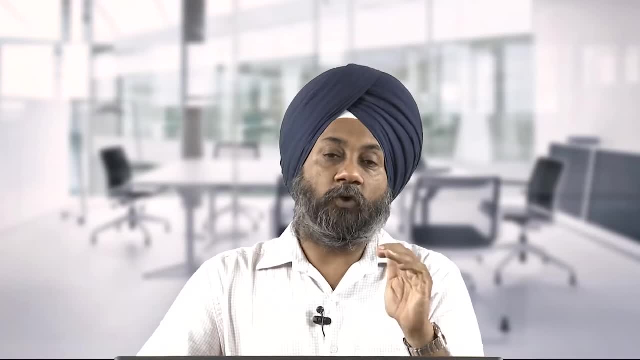 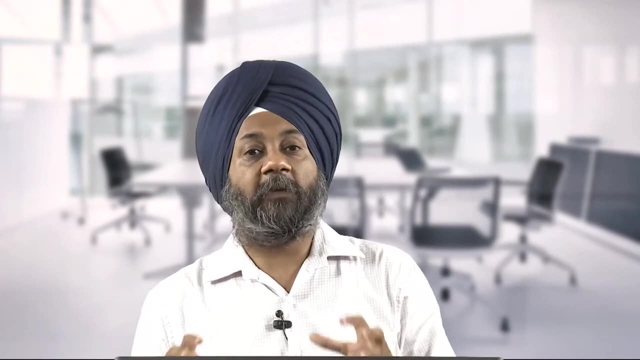 So we have covered a lot many processes And, if you remember, towards the end of our discussion in the 5th week, our topic was design for machining. That if the part has to be made by machining process, what are the guidelines that we must follow? 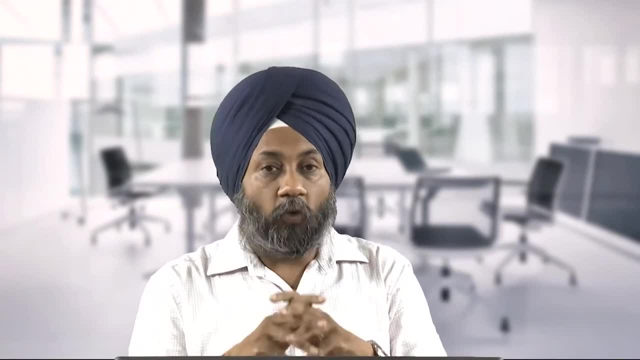 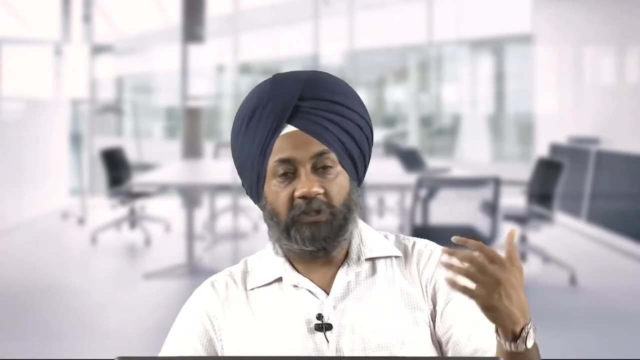 Now you see that we know the guidelines for machining. we know the guidelines for making a product that is forming, giving shape to a product. either it is a metallic product, sand casting or pressure die casting is used. if it is a plastic product, we will be making. 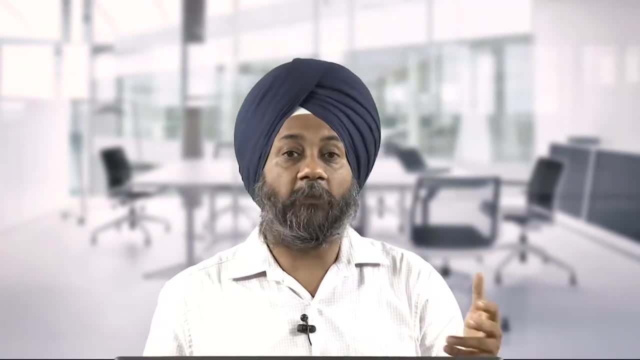 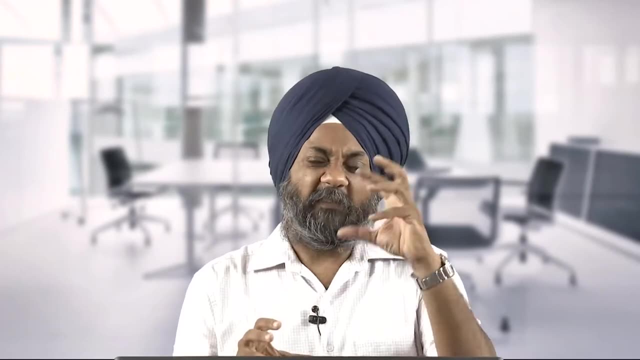 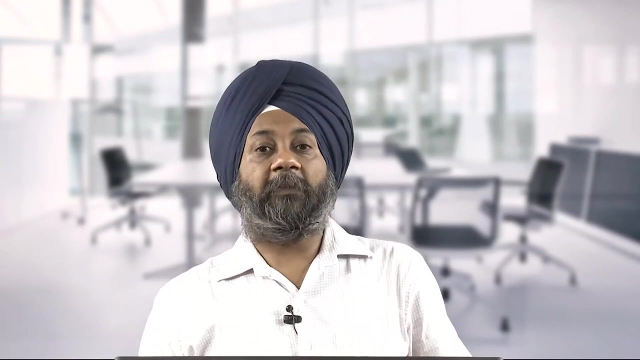 use of. You can very easily relate the processes now: compression, molding, injection, molding, extrusion. So we have seen that how to give shape to a product, whether it is a metallic product or it is a plastic product, and how to cut the product into the desired dimensional accuracy. 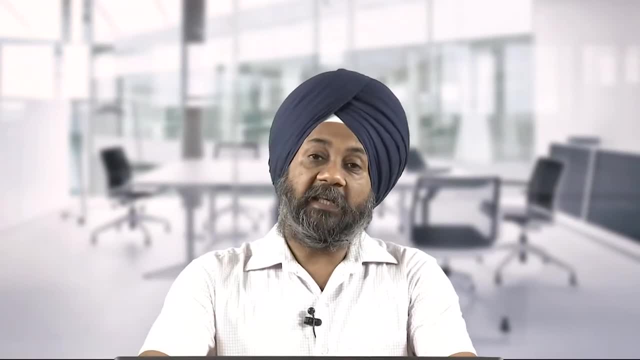 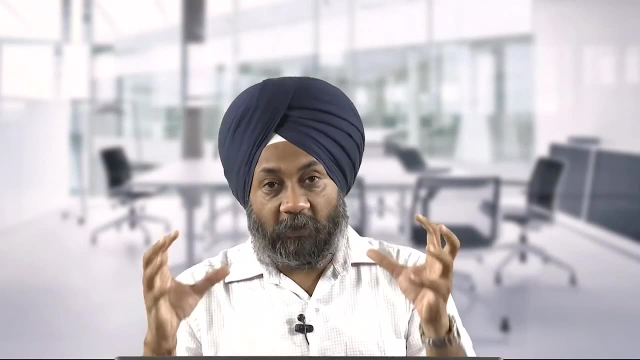 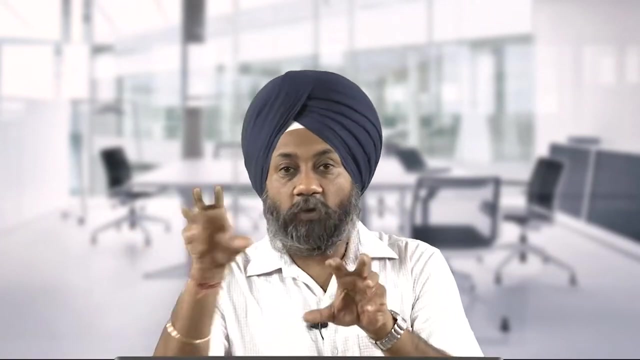 as well as the surface finish. Now suppose in many cases the product is very complicated. so in that case, what we need to do, We need to break down the product into the numbers- Okay, Number of sub parts or sub assemblies- and then we will make these individual parts. 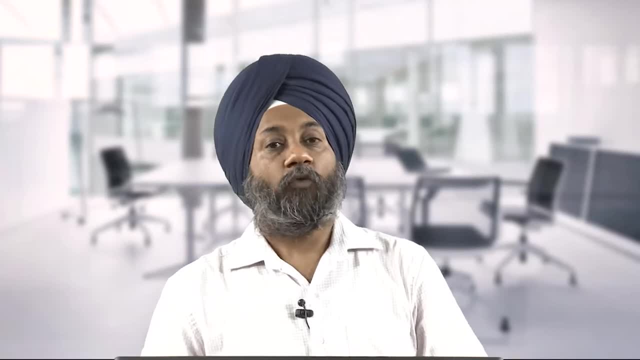 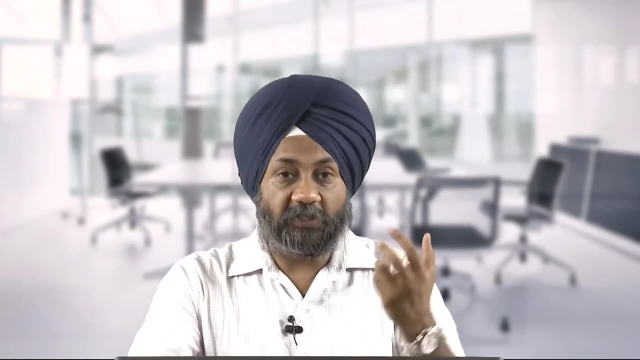 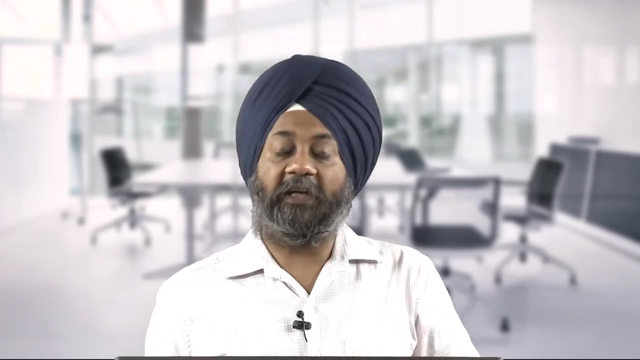 or components and then assemble them together into the final product. So today, our target is to understand the basic intricacies or the basic processes that are used for joining of the various parts, or the processes that are used for joining of the product or assembly of the product. 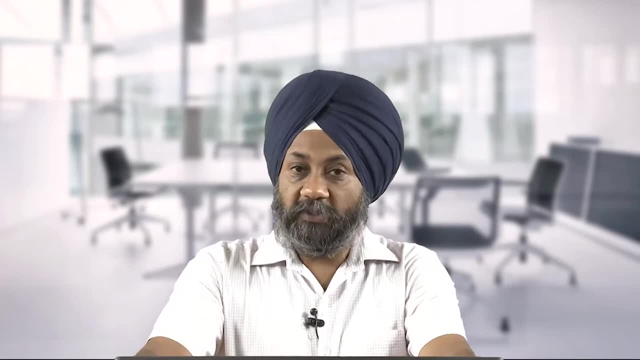 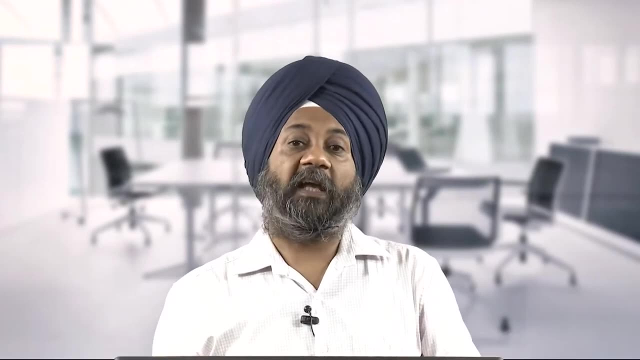 So the word that we are using is the assembly processes. Now, what are these processes? the processes will be using an adhesive. we can have adhesive joining process. we can have mechanical fastening with the help of screws, bolts or rivets. we 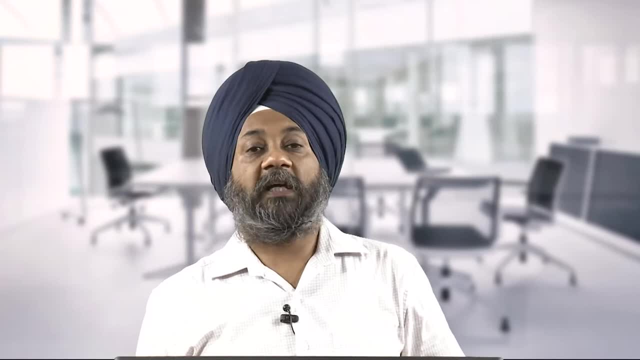 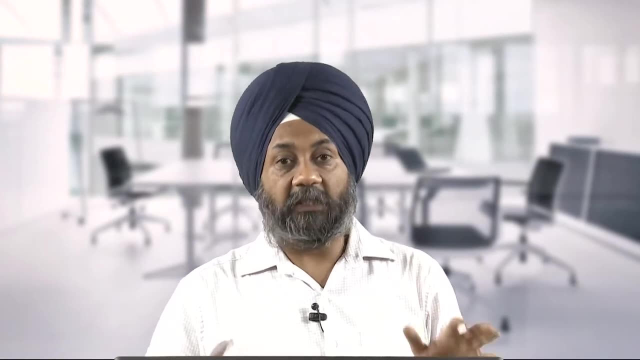 can have welding in which we can have a fusion welding or we can have a diffusion welding, So we can have different types of welding processes. but all the 3- the adhesive joining, the mechanical fastening and the permanent joining- in terms of welding, will help us to. 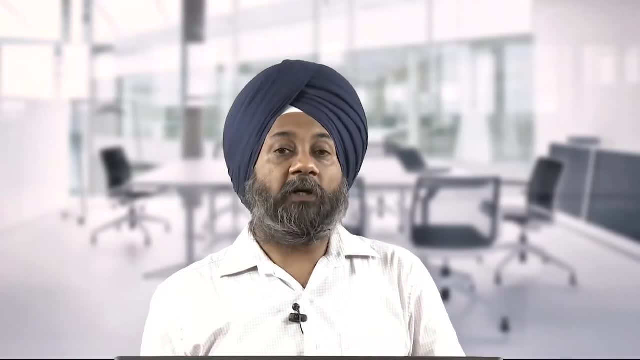 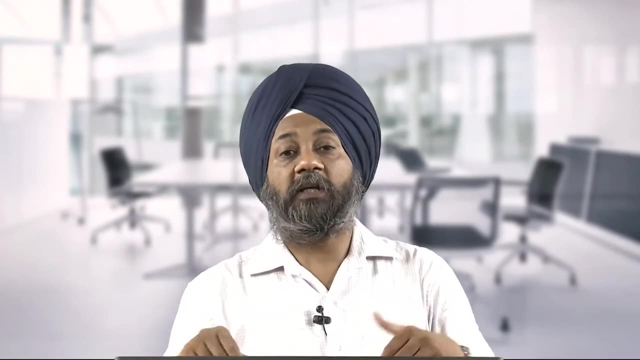 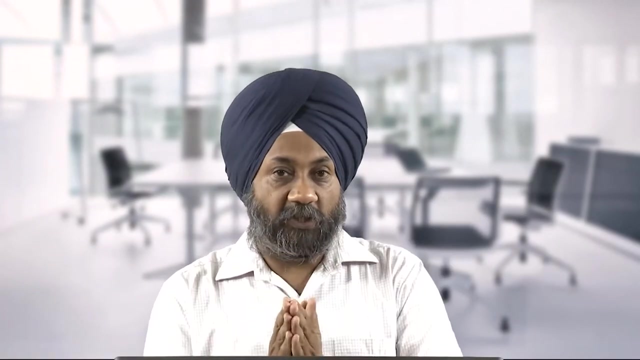 realize a very, very complex product. Okay, A product may be having a very complex geometry which is difficult to assemble. So, in that case, which is sorry, difficult to manufacture using any one standard process, So that product will be made in parts. and these processes that we are going to discuss. 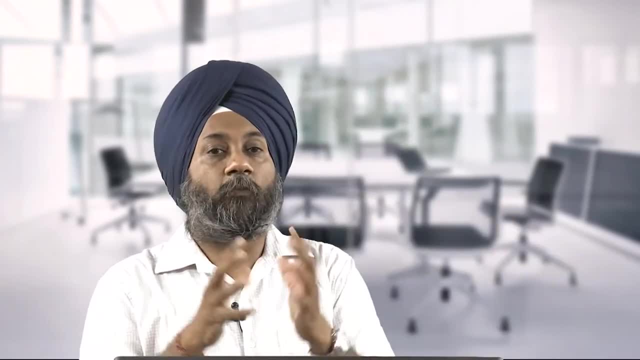 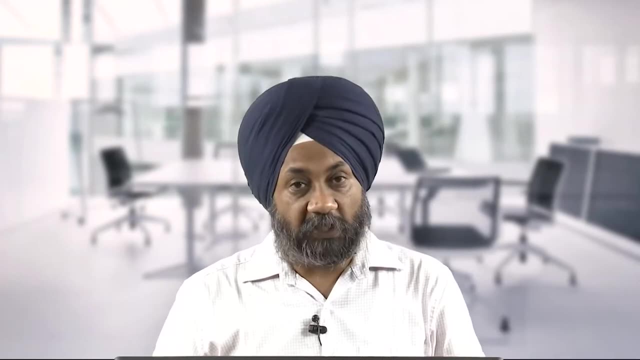 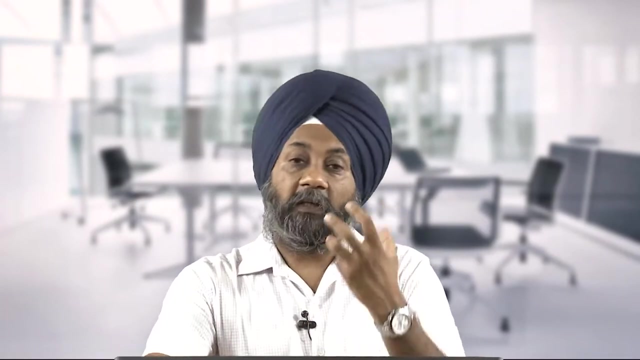 today will help us to assemble these parts or components to get the final product. So, one by one, we will try to understand the basics of the processes and in the subsequent sessions But we will see that how we must design our product so that it is easy to assemble that. 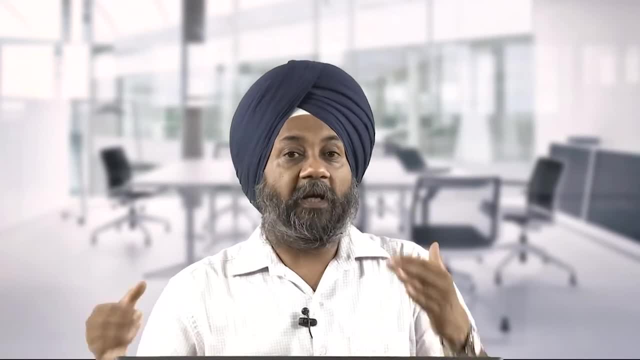 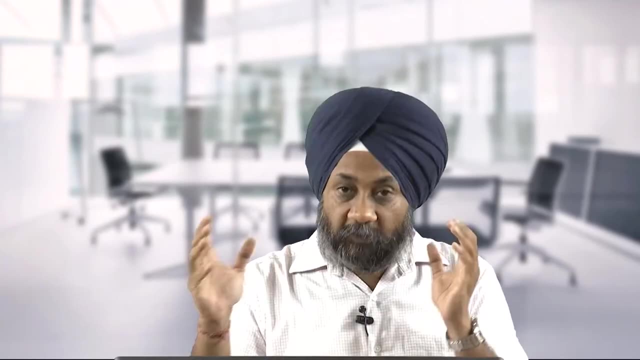 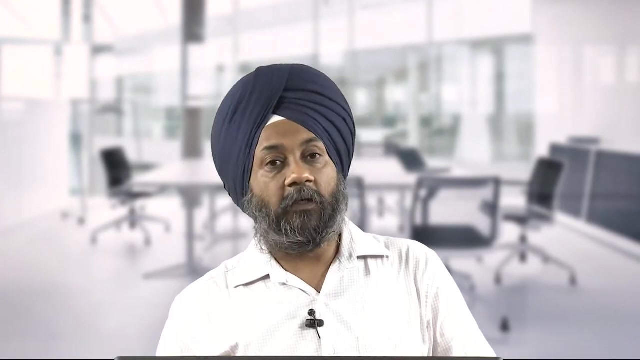 is part number 1.. Then, if the product has to be made by adhesive joining, what product design guidelines we must follow? If the product has to be welded together, with the sub assemblies have to be welded together, what are the guidelines that we must follow? similarly, for mechanical fastening also. 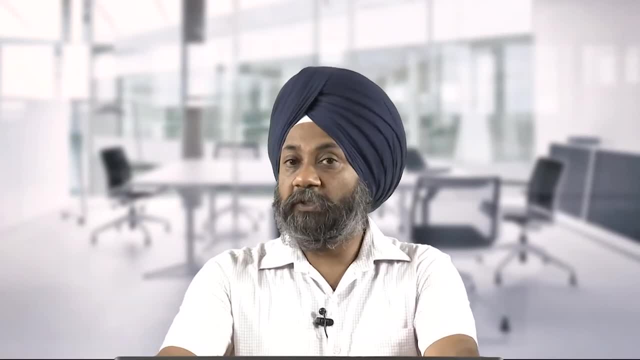 And, if you remember, in the 3rd week of our discussion on this specific topic, We will see that how we must design our product so that it is easy to assemble. that is part number 1.. In the 3rd week of our discussion on this specific course, we have discussed the various 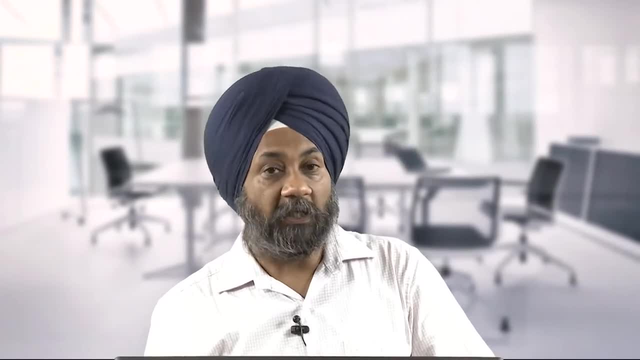 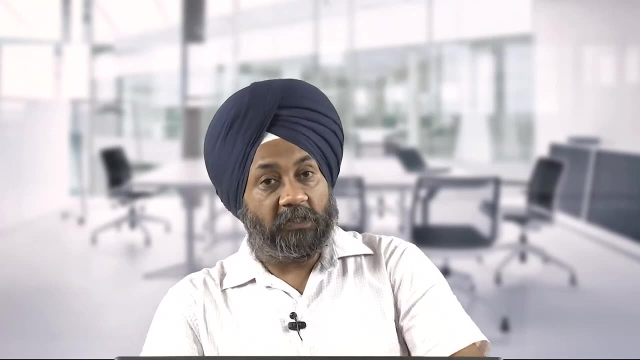 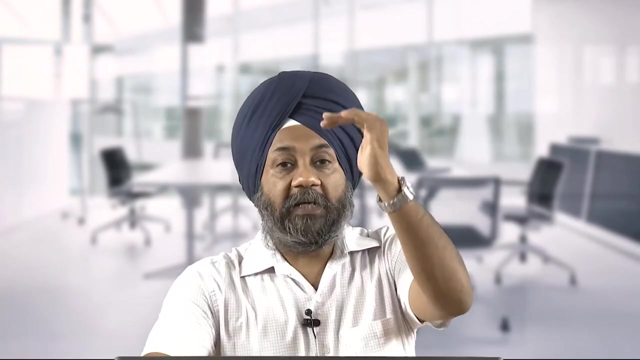 tools and techniques which help us to design the product in the most efficient and effective manner. And there we have considered the concept of design for assembly, which means that we must design our product in such a way that it is easy to assemble. And there were so many DFA guidelines which we must follow during the design of our product. 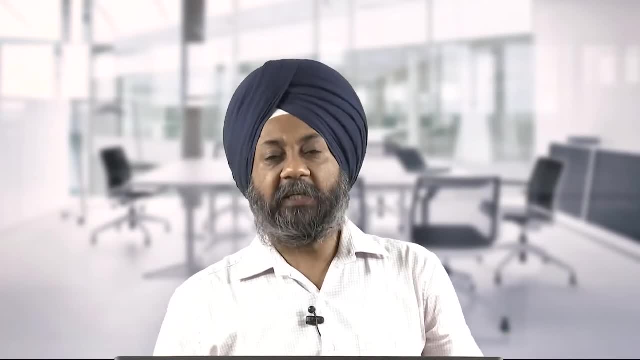 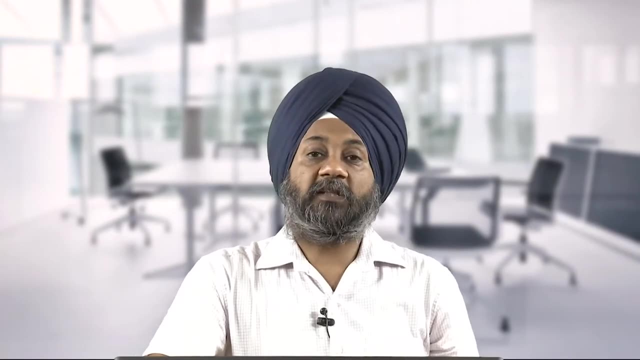 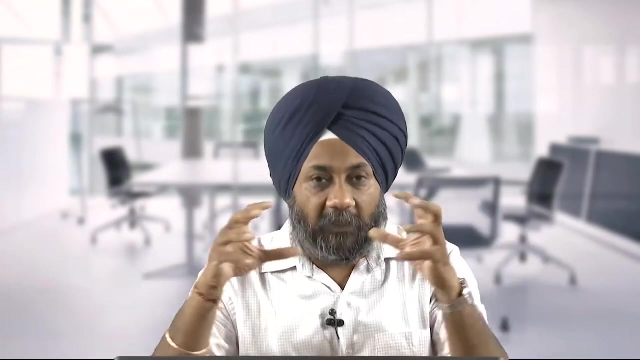 Now, what are these guidelines? These guidelines were related to the DFA. Okay, So DFA is the top down type of assembly approach. minimize the part count, that is, number of components must be minimized. then ensure modularity in design or ensure the modular design. combine the parts wherever possible. 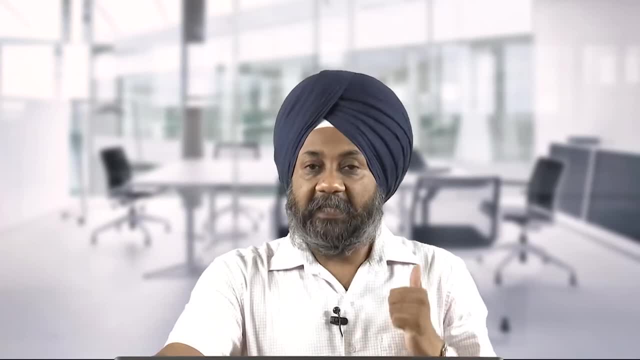 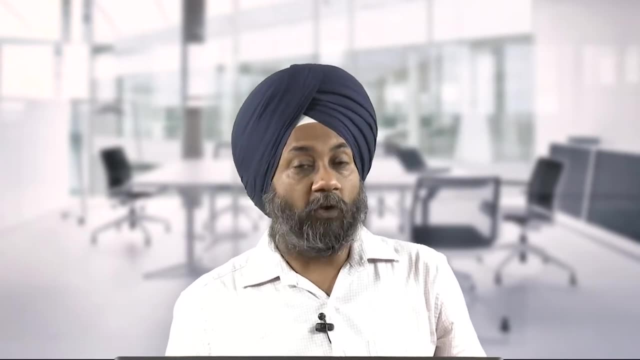 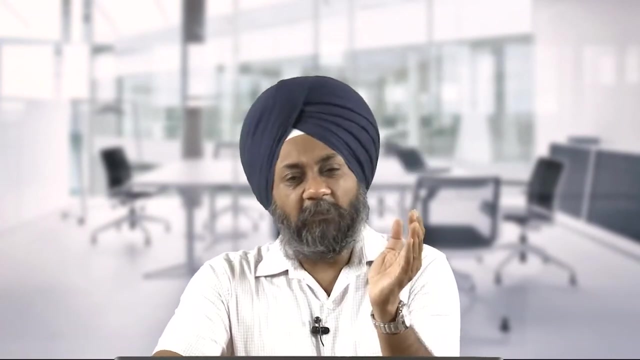 So there were number of guidelines which fall under the DFA. So what is DFA? let us start today with our discussion for DFA- that when we are designing a product, we must keep in mind that the product must be easy to assemble. Okay, And when we have designed the product with minimum assembly operations, then how to do? 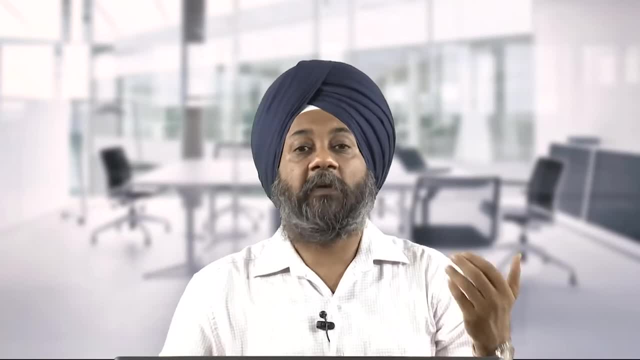 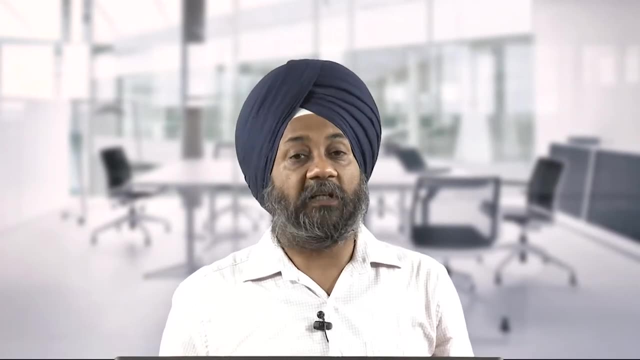 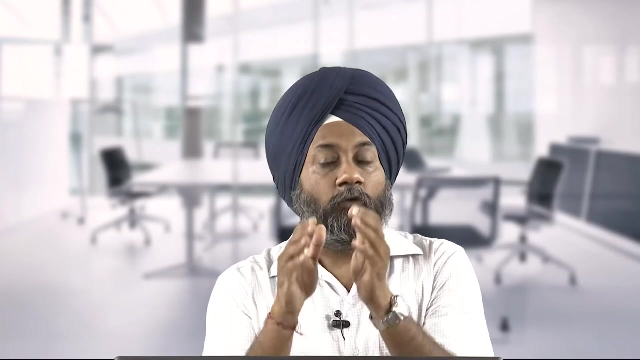 the assembly that is the subsequent part of today's session, maybe by using adhesive joining. So where adhesive joining is applicable, we will try to see. where mechanical fastening is applicable, we will try to see. where welding is appropriate, we will try to understand. So, before going to that where we will only follow the assembly or the joining processes, 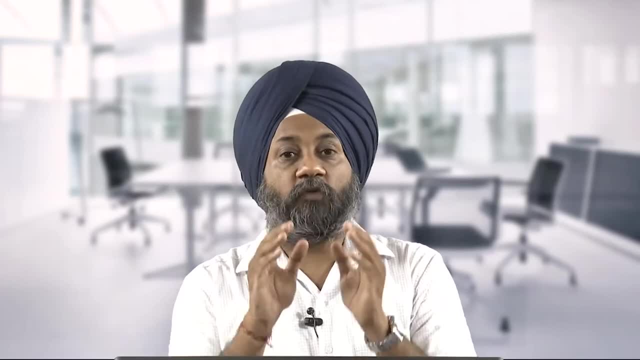 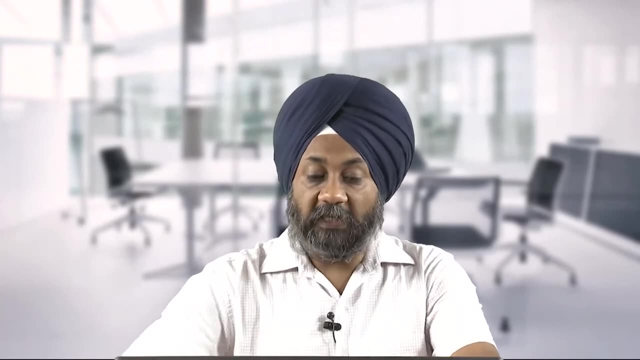 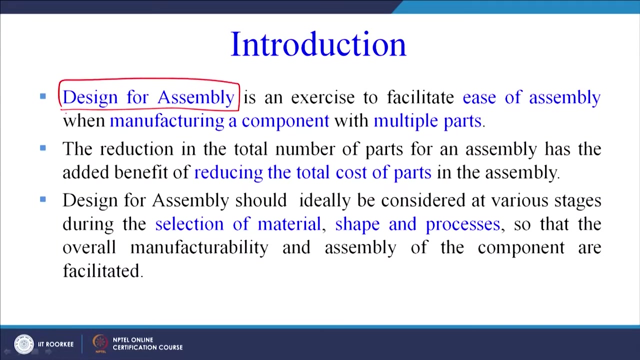 wherever they are necessary. First and foremost, we must try to make the modular part where we have minimum requirement of the assembly processes and that is in line with the design for assembly which we have already covered. So for, in design of assembly, what do we do? so DFA design for assembly is an exercise. 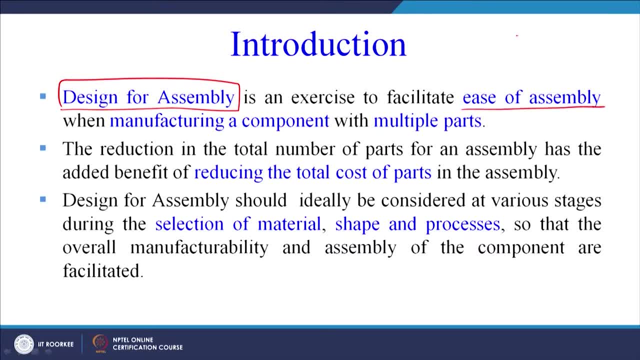 to facilitate ease of assembly. So when we are designing a specific product, for example, we must try to design it in such a way That it is easy to assemble with the other part. So the design guidelines must be kept in mind during the design stage only. 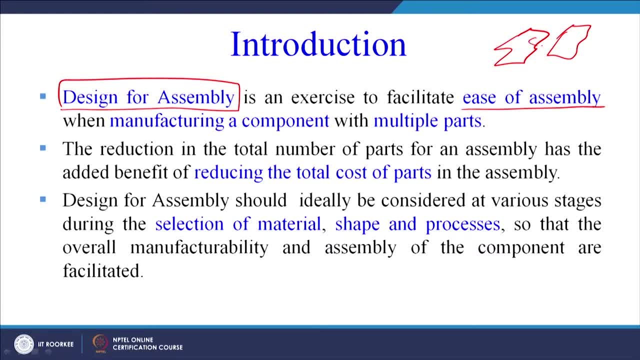 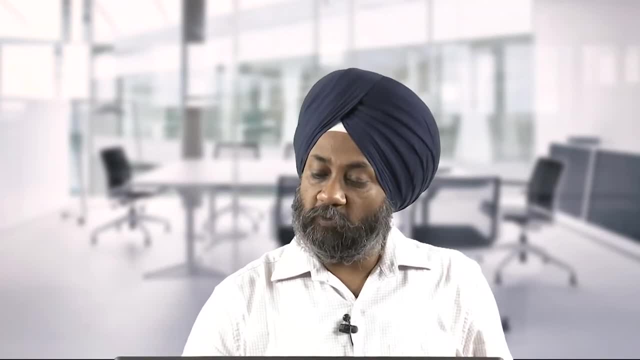 So design for assembly is an exercise to facilitate ease of assembly between the different parts when manufacturing a component with multiple part. So wherever multiple parts are there, we must design the product in such a way that it is easy to assemble. first and foremost, we must also try to reduce the multiple parts by using 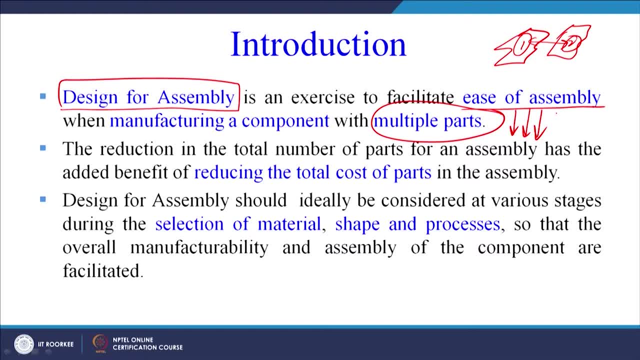 the redesigning the product. The reduction in the total number of parts for an assembly has the added benefit of reducing the total cost of parts in the assembly. So we will reduce the cost of parts when they are going to be assembled together If we are able to- if, as I have already mentioned here- reduce the number of multiple parts. that 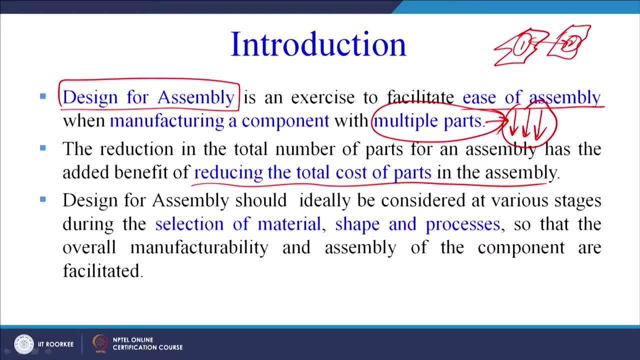 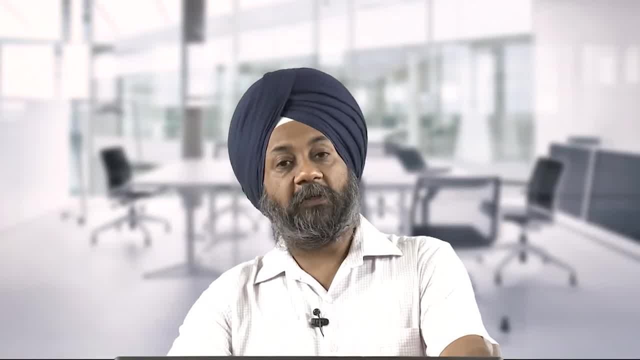 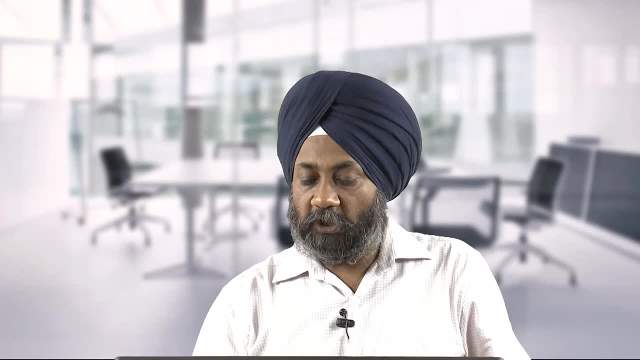 go into the assembly. Design for assembly should ideally be considered at various stages during the selection of material. So when we are selecting the material, we must be very, very cautious regarding the DFA guidelines, because the parts have to be finally assembled into the final product. 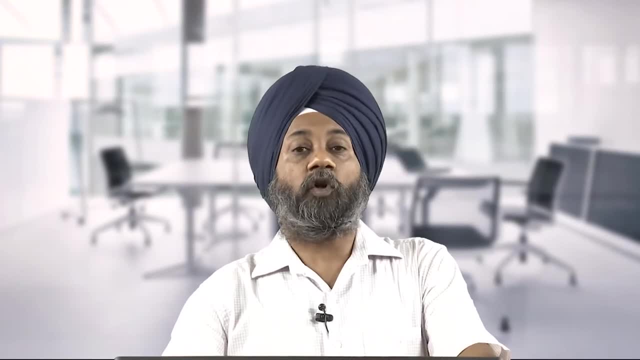 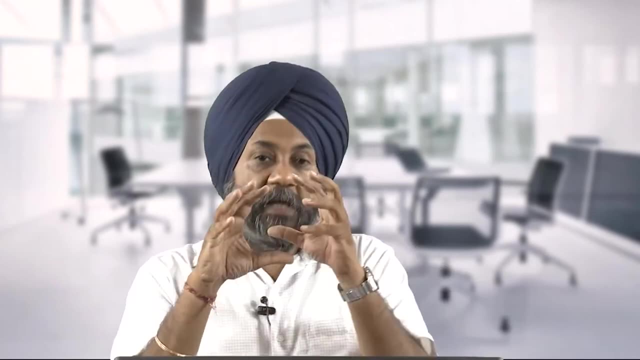 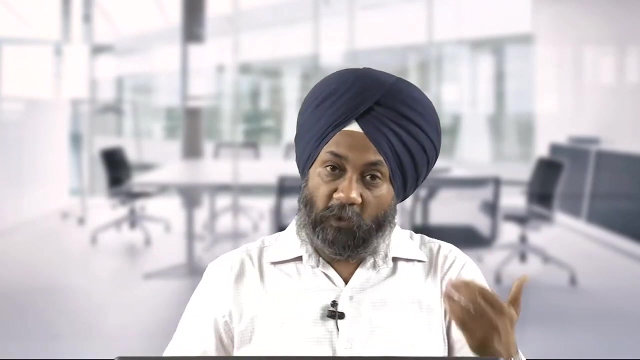 Shape and processes that we are going to use so that the overall manufacturability and assembly of the component are facilitated. So, overall, our objective is to make the product with the minimum manufacturing cost and for that we have to keep in mind all the guidelines: the design for manufacturing guidelines, the 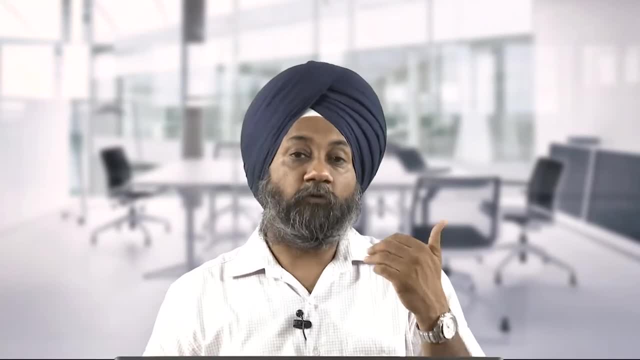 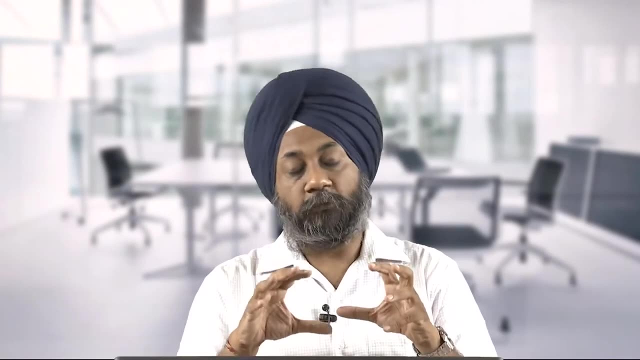 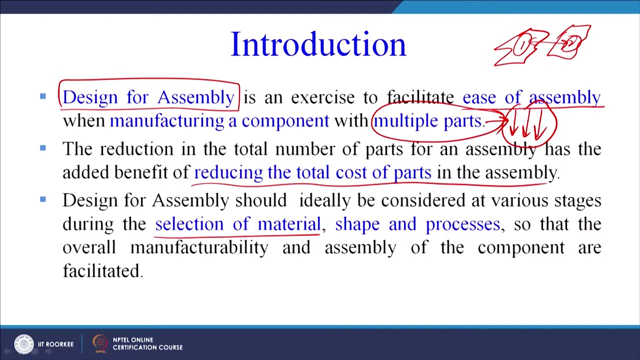 design for assembly, guidelines, guidelines, the design for safety, design for reliability, design for production, design for manufacturing, manufacturability and assembly. So there are number of different types of- and I must add the word conflicting- guidelines. why conflicting? because of one of the guidelines, or by following one specific guideline, we 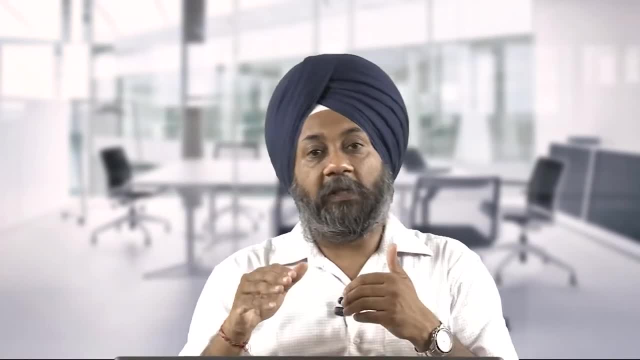 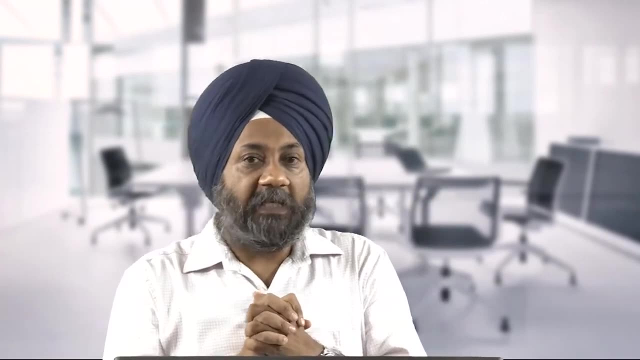 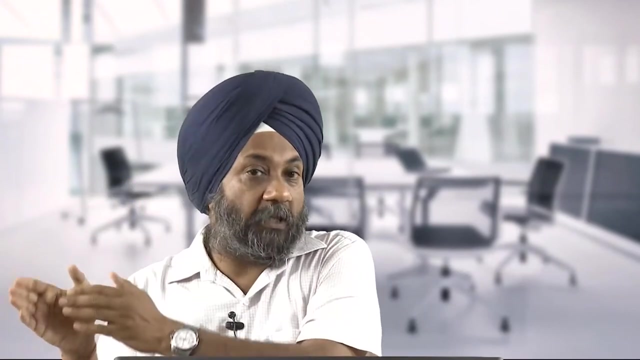 may be transgressing into or we may be violating some of the other guidelines. For example, if we religiously follow the design for manufacturing guidelines, we may be violating some aspect of design for assembly guidelines. and if we religiously follow design for assembly guidelines, we may be violating some of the basic principles of design for. 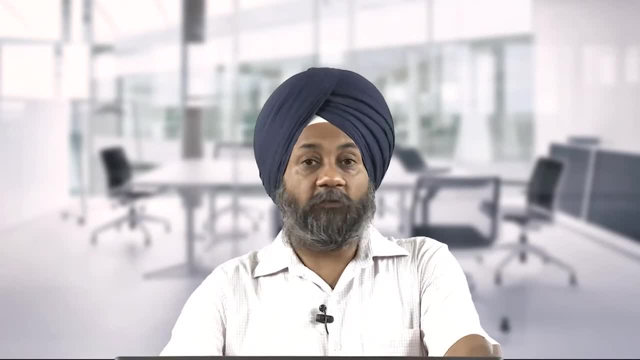 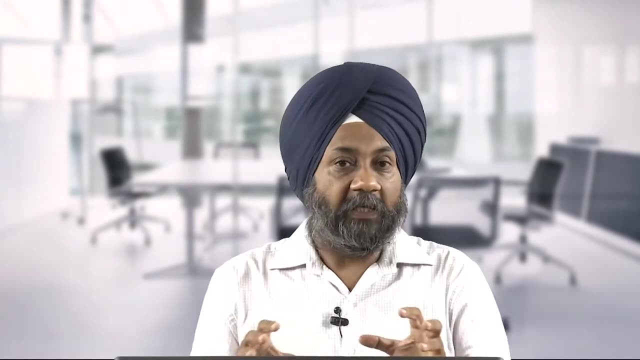 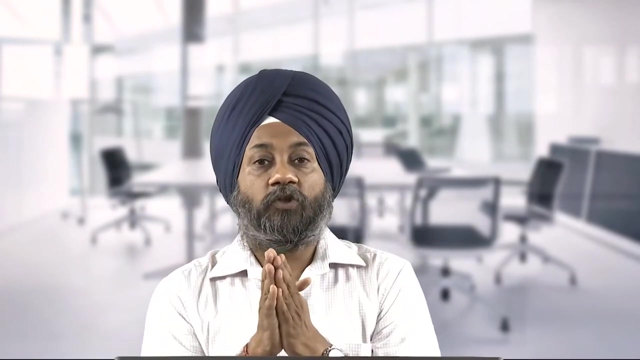 assembly, which we have already understood during our third week of discussion. So, overall, to ensure the manufacturability of our product, we must keep in mind that the joining processes must be limited to a very less Number, because if you have lot of joining processes to be done, the cost of the product 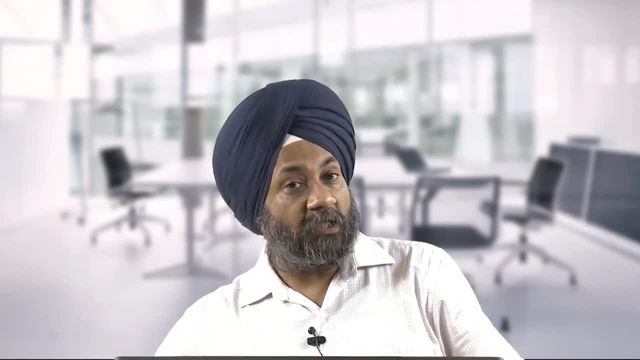 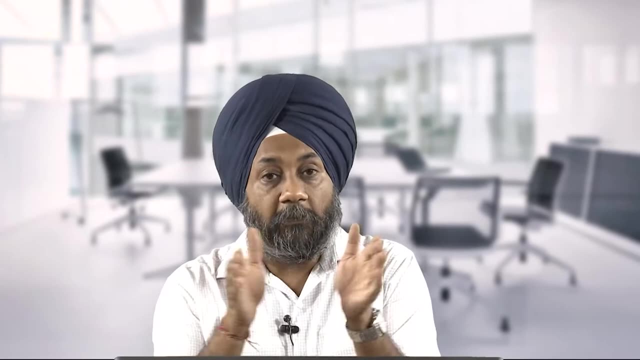 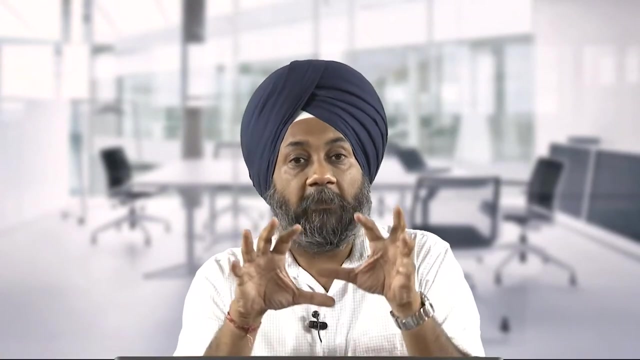 will definitely go high and therefore you will see that in most of the design these days, we talk about modularity, we talk about modular designs with minimum requirement of assembly. So the first and foremost thing that we must keep in mind is that we have to minimize the 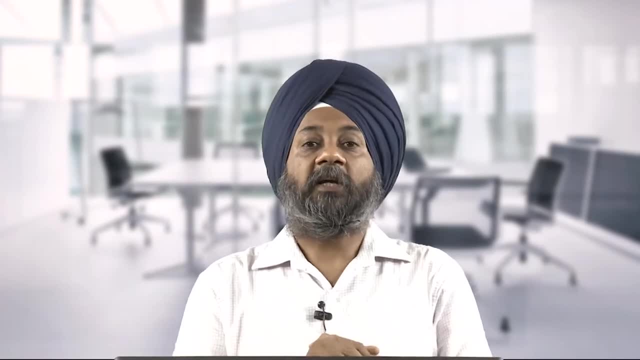 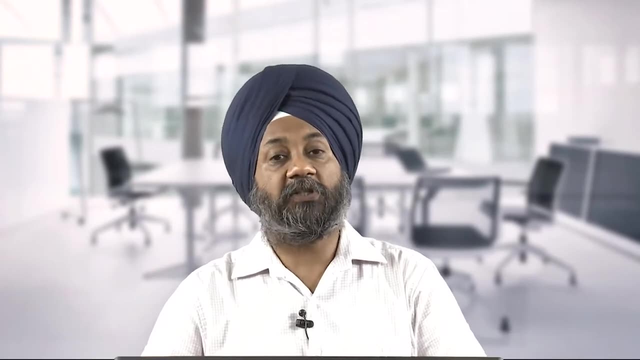 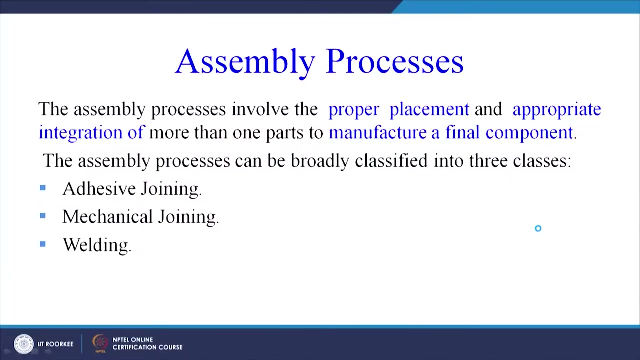 number of parts which need to be assembled together to get the final product And, in case the assembly operations are required, what are the processes that we are going to study in the subsequent slides? So the assembly processes. you can see the assembly processes involve the proper placement. 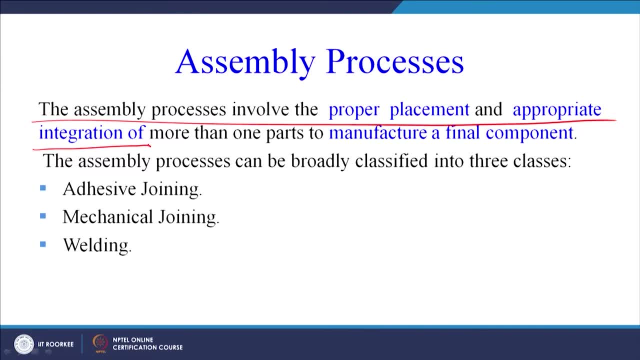 and appropriate integration of. so we have to ensure that the 2 parts which need to be joined together are placed properly, and appropriate integration of more than 1 parts to manufacture a final product. So our final component is the final product that we plan to produce. so assembly processes. 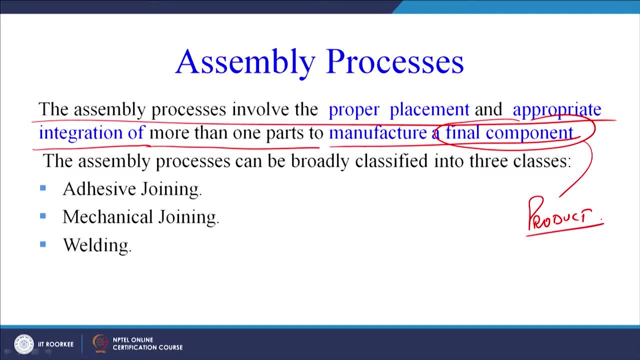 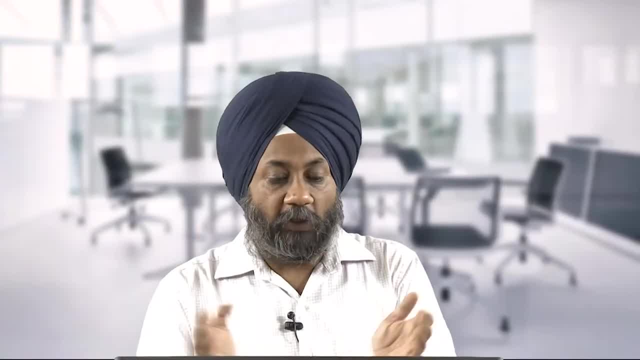 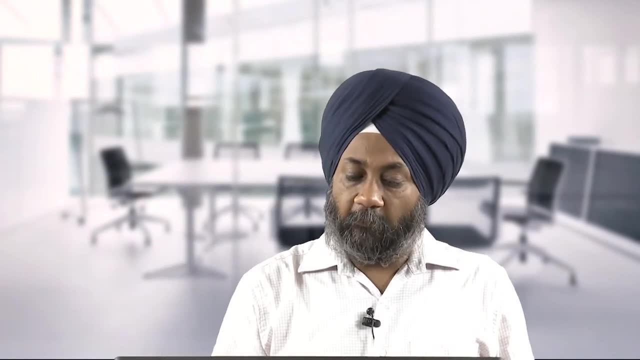 will involve the proper placement and integration of more than 1 parts. Now this word integration, if in mathematics also we see we add up, so integration means we are trying to integrate 2 or 3 different parts together. so the assembly processes can broadly be classified into 3 classes. 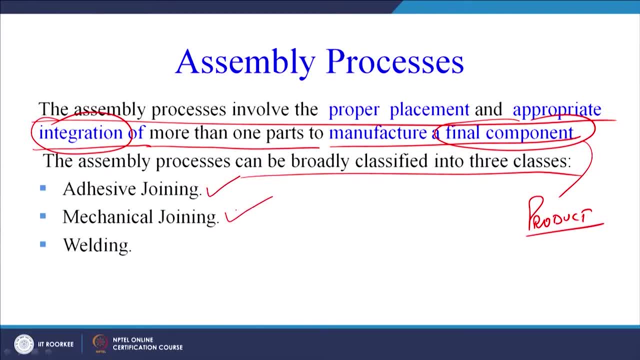 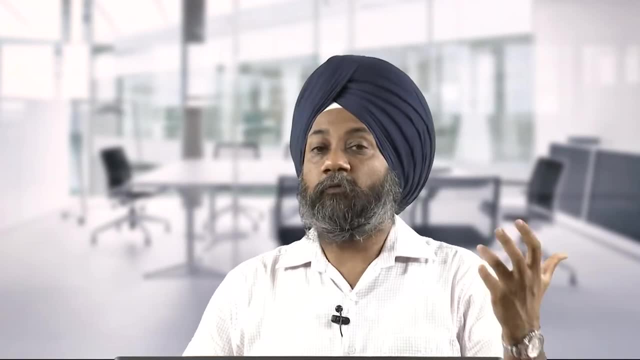 So we can see adhesive joining, mechanical joining and welding. so most commonly we see from mechanical engineering point of view and joining of metallic parts we take undertake different types of welding processes. So if the product has to be manufactured and if we talk about- usually I take the examples. 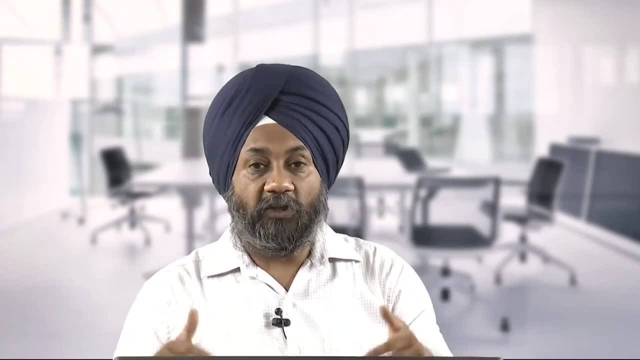 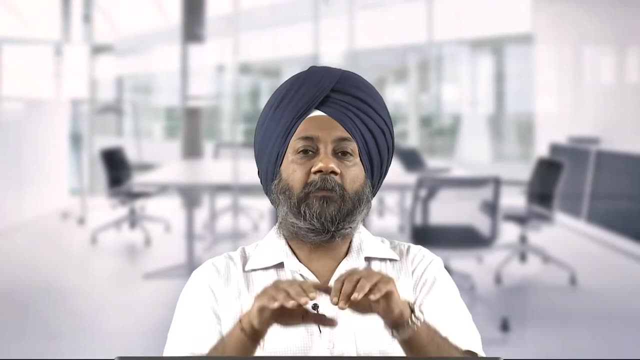 from our day to day life. If you talk about the camera that is recording this video or which is recording this session, the camera is a highly complex part And there may be 100 or 150 parts that I can see, which may have been assembled together. 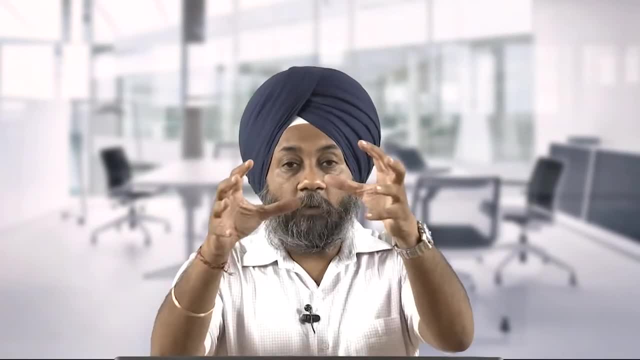 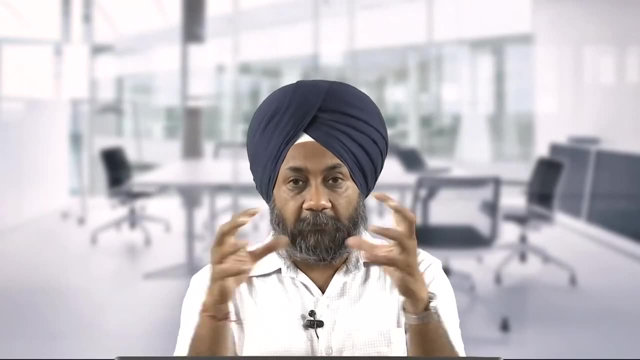 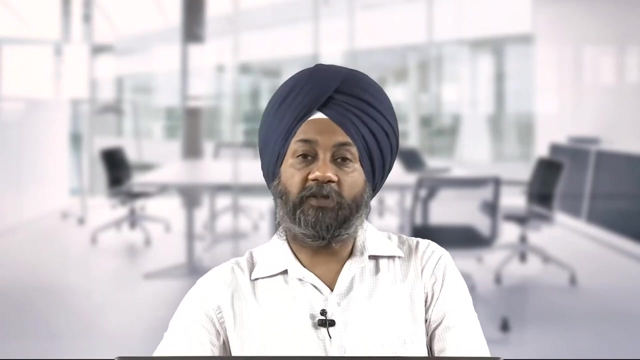 to bring this overall product into picture. so the overall product is our camera. But number of assembly operations have been done. number of different parts of different materials have been joined together, assembled together to make this product. so we cannot undermine the importance of assembly operations, specifically in case of product design. so 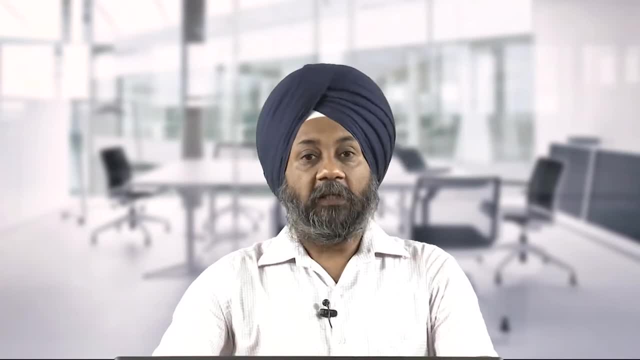 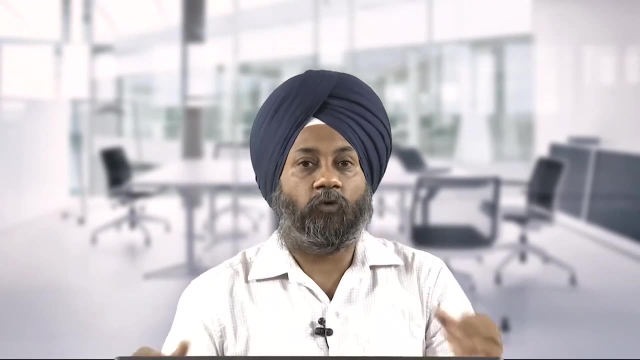 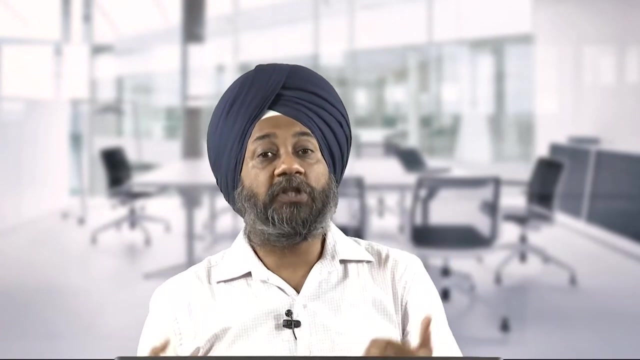 when we are designing a product, We must ensure that how the product is going to be finally assembled, what are going to be the sub parts and how this sub parts have to be integrated, and many a times we may not be really interested that the user may be able to see the joints. 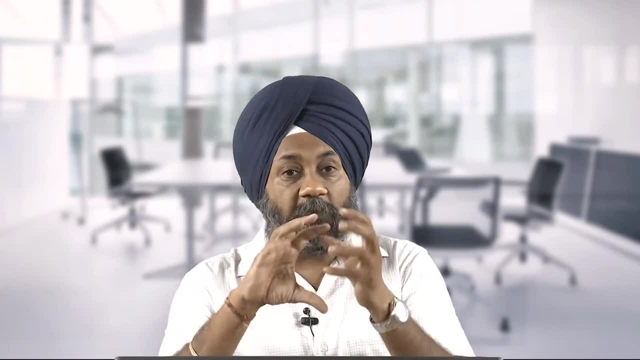 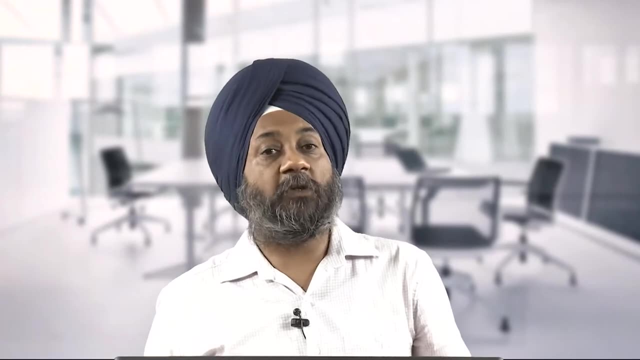 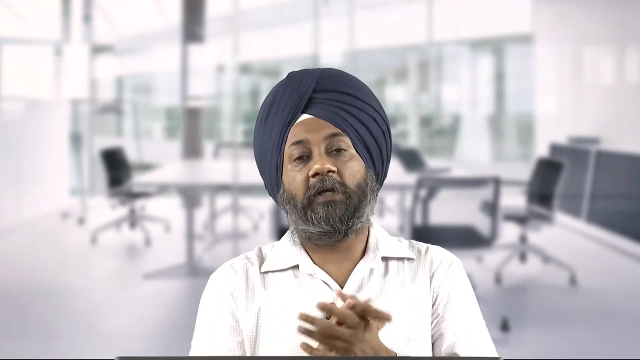 So we need to sometimes camouflage or sometimes cover the joints in such a way that the user is not able to comprehend that how the product has been joined together. So the joining Approach or the joining methodology that is going to be adopted is very, very important. 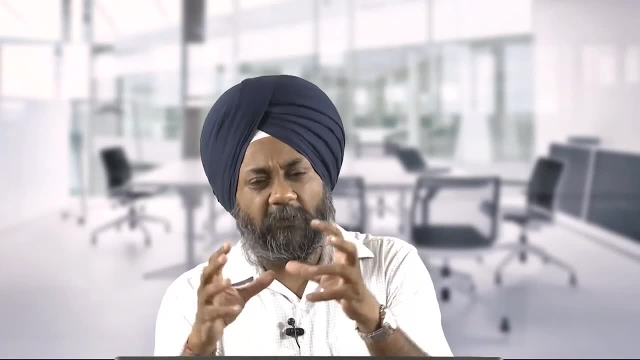 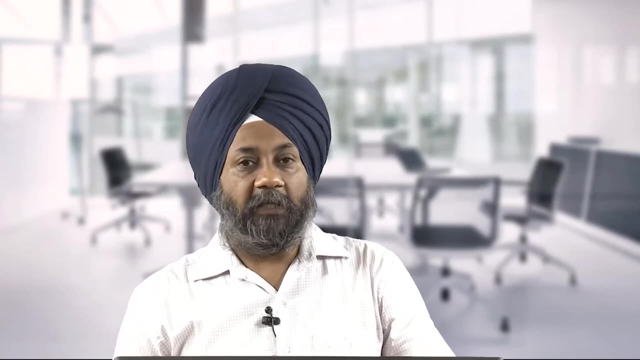 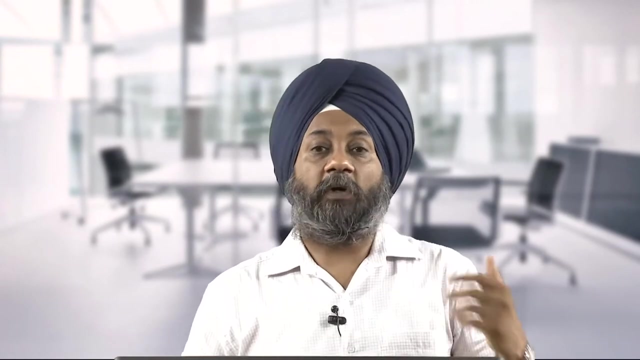 and it cannot be just like that that we design a product and when we start assembling the product, we are not able to assemble it properly. why? because we have not understood the complexity in the assembly, as well as we have not given due attention to the joining processes during. 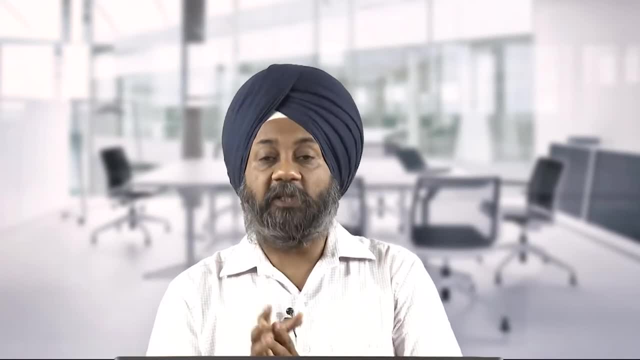 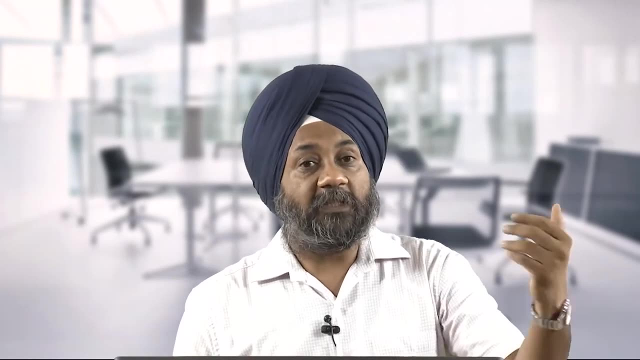 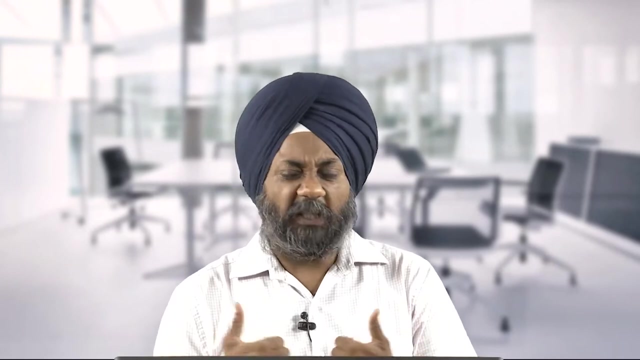 the product design process And Therefore This process is very, very important. what is the versatility of the process? how it can be applied, what are the specific areas where this can be applied? so all that we need to understand. So today is an introductory talk about the assembly processes and in subsequent sessions, 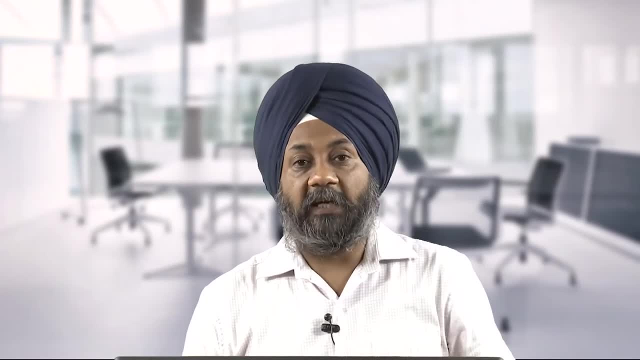 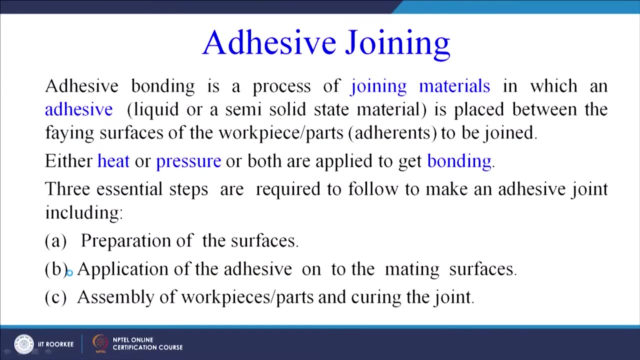 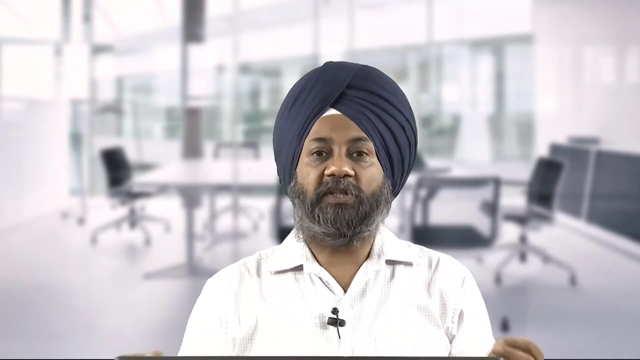 we will talk about in detail that. what are the product design guidelines for the specific processes? So the first one is the adhesive joining. and again I am going to take an example from our day to day life, In our daily life for our children, if a toy is broken, we usually try to fix it using any 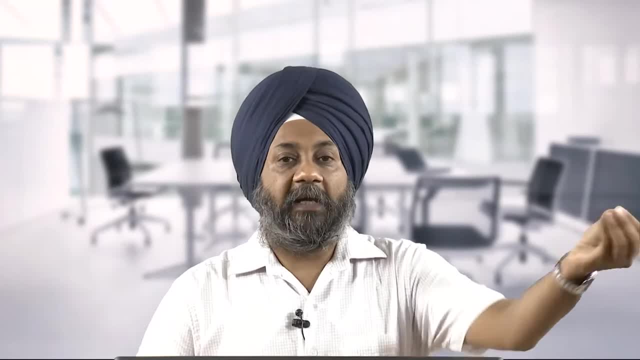 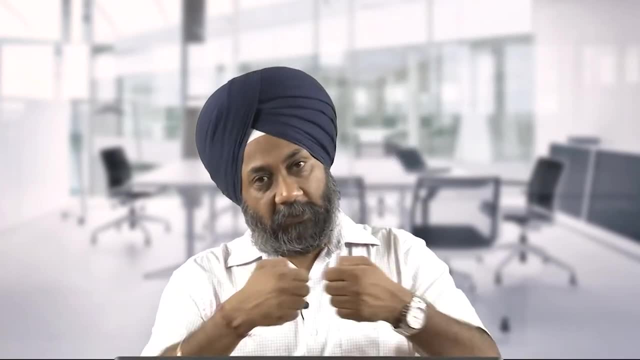 standard adhesive which is available in the market. So we go and buy adhesive, bring the 2 parts together, do some surface preparation and apply the adhesive. leave it for maybe a day the product is joined, or the product that is in this case is a toy is joined. 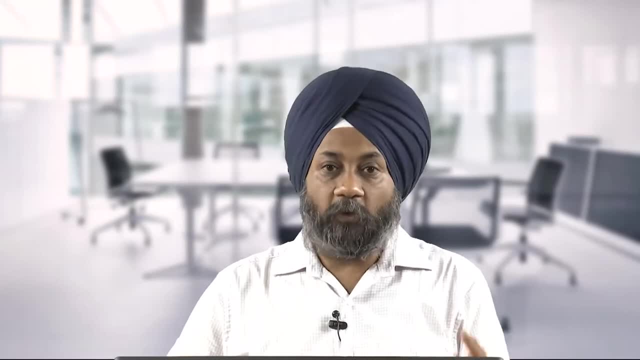 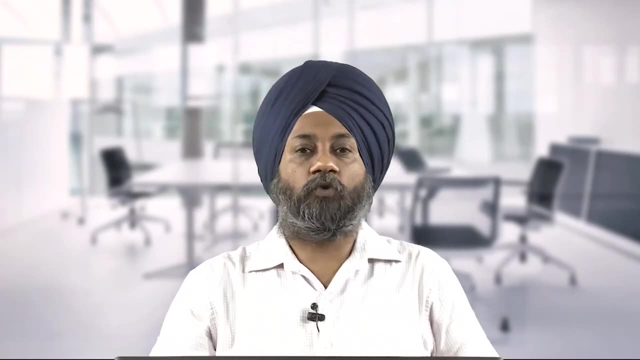 So that is a very simple example of adhesive joining. normally we do. we take our shoe. the sole has come out, We take it to a cobbler. The cobbler applies adhesive and then fixes the 2 parts together. that is an example of 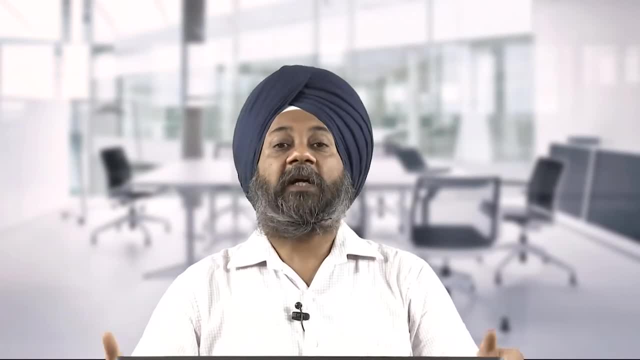 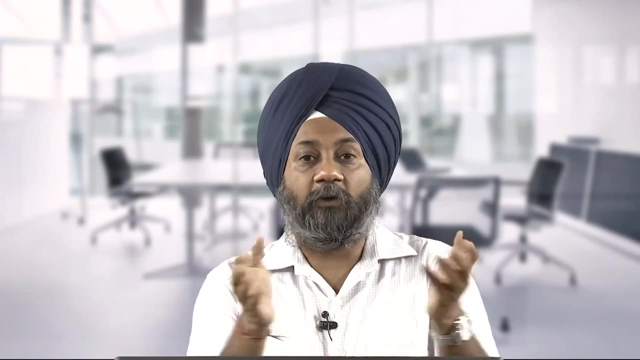 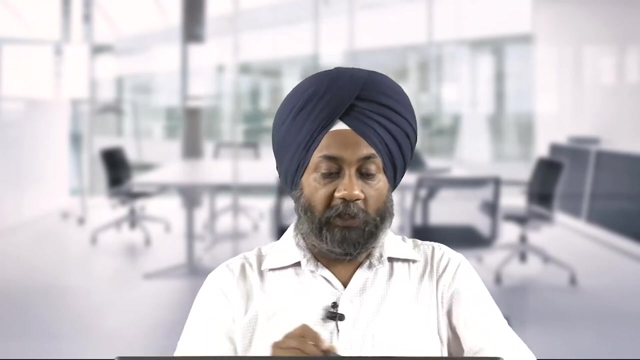 adhesive joining in our day to day life, But adhesive joining is also used for engineering structures, for engineering products. and what is adhesive joining? if you have understood the example, I do not feel that you will feel any problem understanding what is given in this slide. So you can see that adhesive bonding, either process of joining materials, now materials. 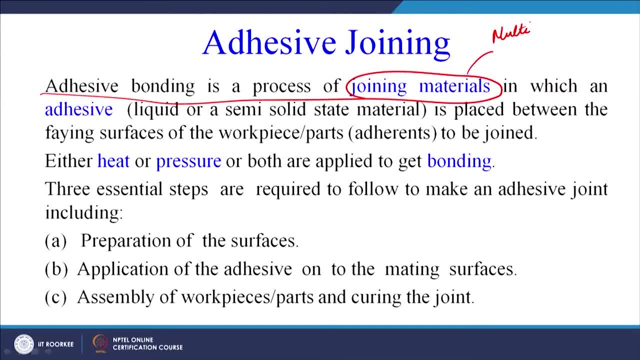 can be multiple materials also, So normally we use the word adherent for the material that is to be joined. So the adherents can be of different materials. you can join wood plus another part can be made in plastic, or it can be metal or a wood. 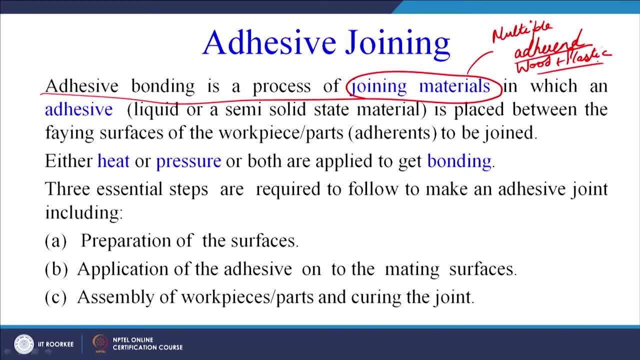 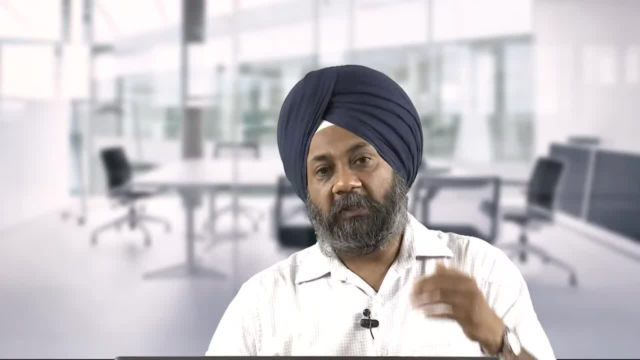 So you can have different types of adherent. So adhesive joining is a process of joining materials, in which an adhesive, which I have already told It- is a polymer that we use for joining the 2 parts together, which can be in a liquid or a semi-solid state material. 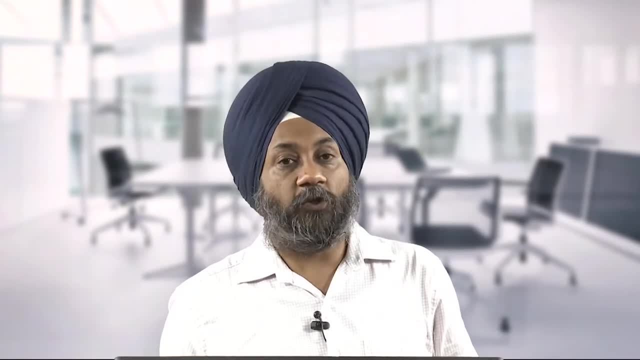 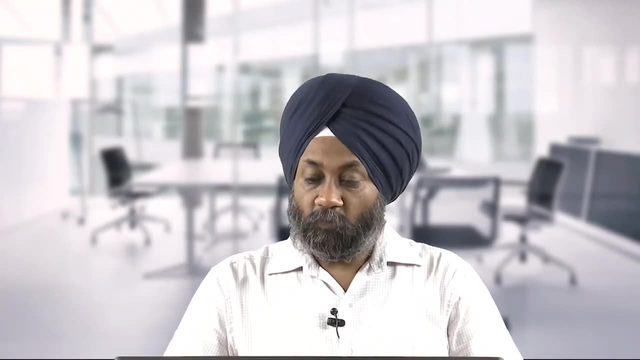 If you go to the market and you buy adhesive to join the toy which is broken, you will see that it will be in a semi-solid or a viscous state, So liquid or a semi-solid state. So the adhesive is placed between the faying surfaces. 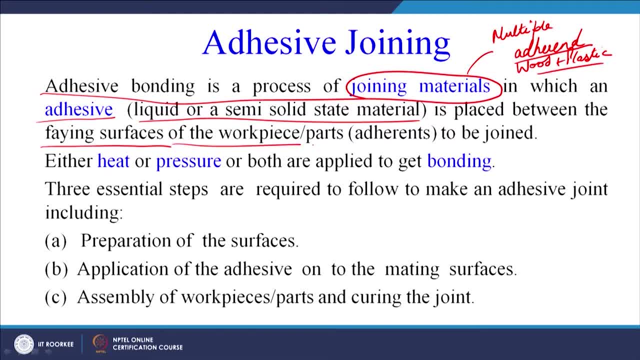 The surfaces to be joined together of the work piece or the parts which is given adherents to be joined. So this is the word that I have used, This is the word that I have already mentioned here. So these are the adherents that we need to join together. 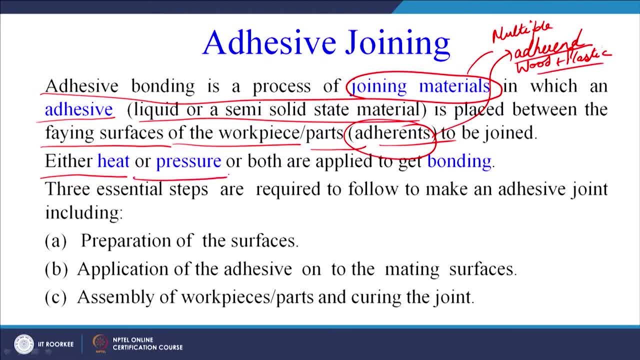 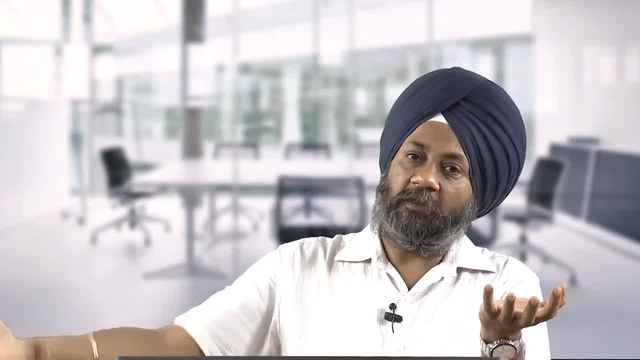 Now either we will apply the heat or we will apply the pressure. Sometimes, when we have to join the 2 pieces together, we put the adhesive, we join them and then we keep some weight on top of these 2 layers that we have joined. Why do we keep the weight? 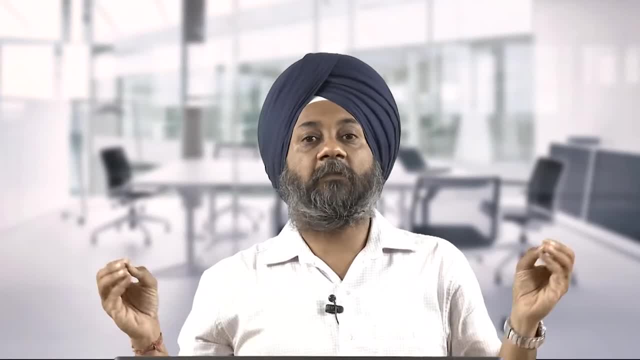 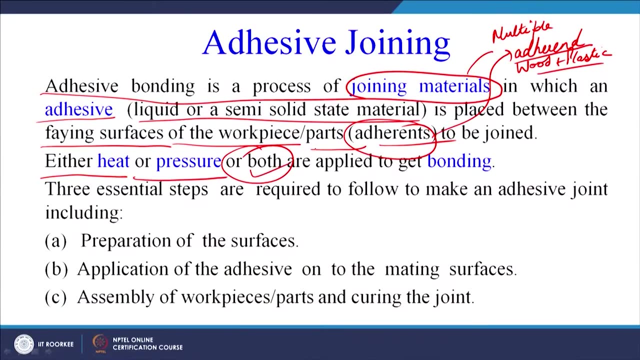 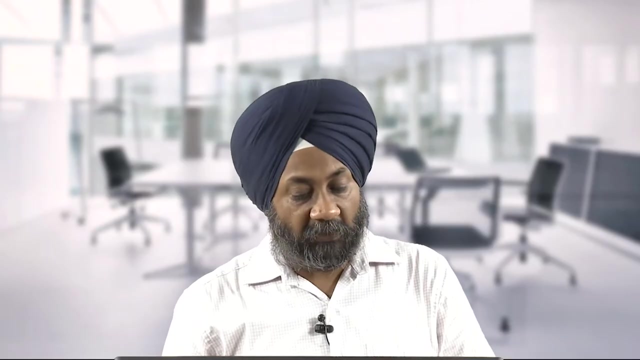 So because that is applying the pressure and in some cases we may supply some heat also. So either heat or pressure, or Okay, Both are applied to get the perfect bonding between the 2 work pieces or the 2 adherents that we want to join together. 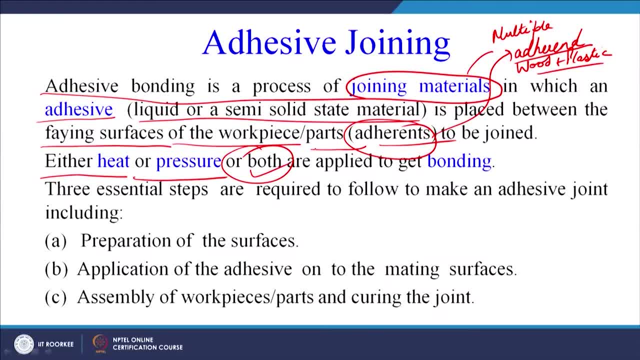 Three essential steps are required to be followed to make an adhesive joint. Now these are the 3 step process and specifically the adhesive joining. First one is preparation of the surfaces. The surfaces may not be that smooth. Suppose this surface. I want to join with this surface. 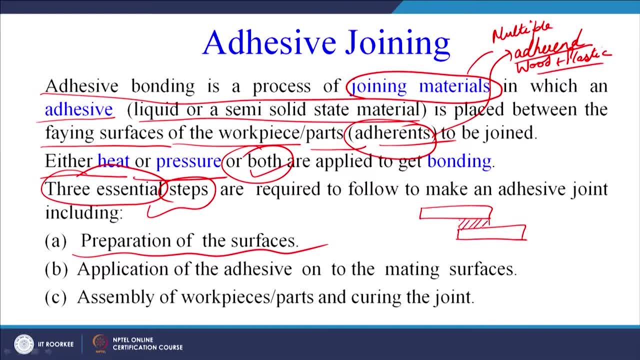 This is my overpass. This is my overlap area where I want to apply the adhesive. Now, these 2 surfaces that I am joining may not be ready to be joined together, So first thing is we need to do the preparation of these 2 surfaces. 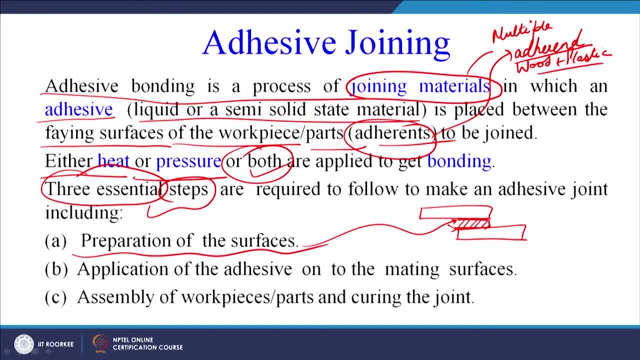 Application of adhesive on the mating surfaces. So we have to apply the adhesive here, as I have shown with the thicker line. Assembly of the work piece part and curing of the joint. Now curing is the process for the polymers in which they become solid. 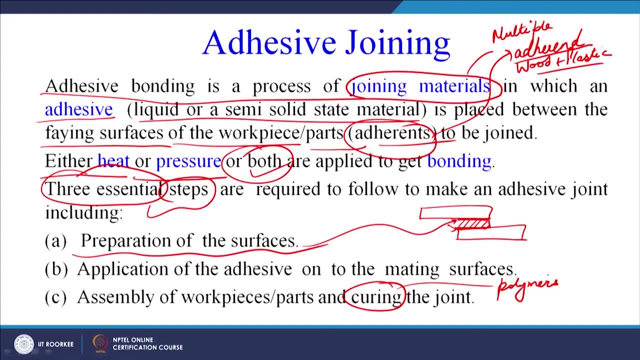 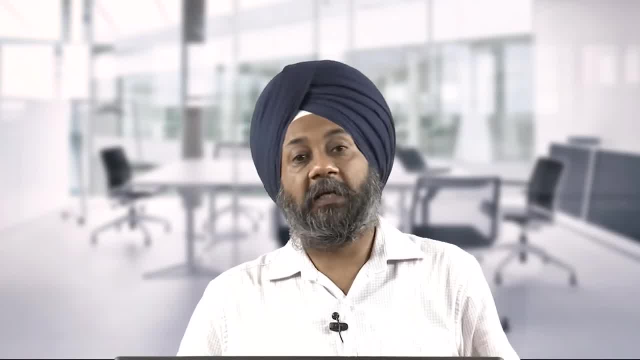 Solid from the semi-solid state. So that is the very basic definition of curing process. otherwise, if you want to understand curing, you have to understand it from the chemical or the chemistry point of view, or the chemical engineering point of view, where we talk about thermosets. 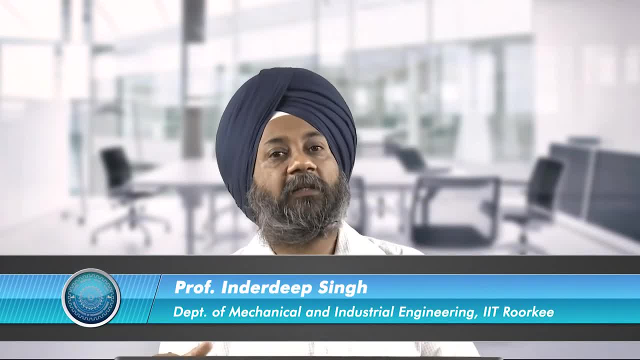 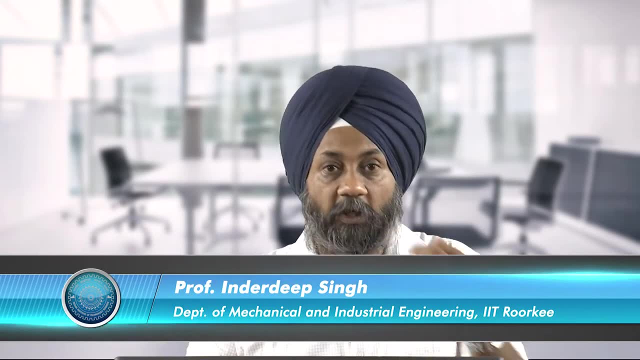 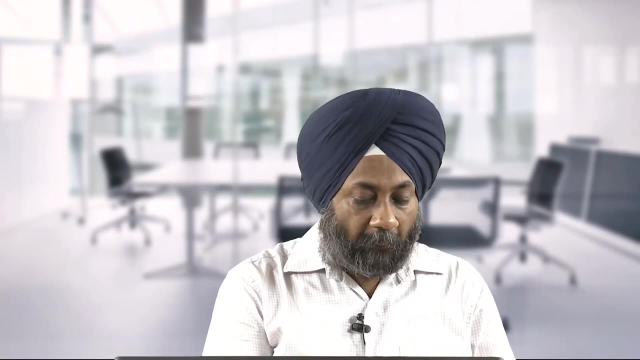 We add a hardener into it and then there is a reaction and then the 3 dimensional molecules are formed, or network of molecules is formed, which led to the solidification of a polymer. So we are not going into that much detail, But we are going to understand that there are 3 steps which a product designer must. 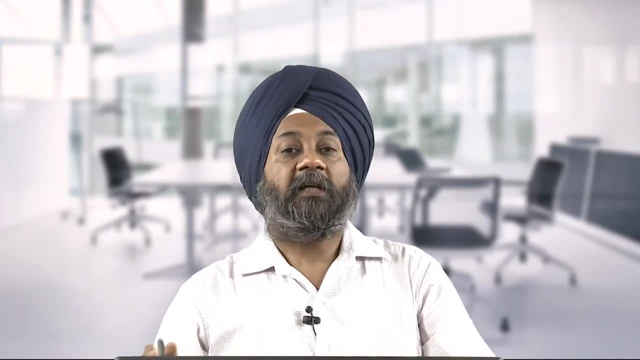 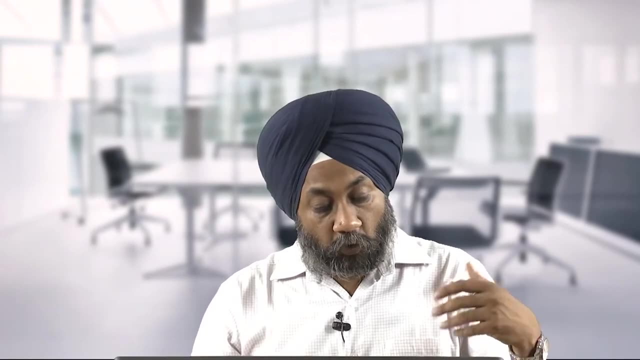 keep in mind when the product is designed So that the surfaces can be prepared to be joined by adhesive joining. So this is, these are 3 steps, which is absolutely clear. preparation of the surface: sometimes surface is very, very smooth, very difficult to join using the adhesive. 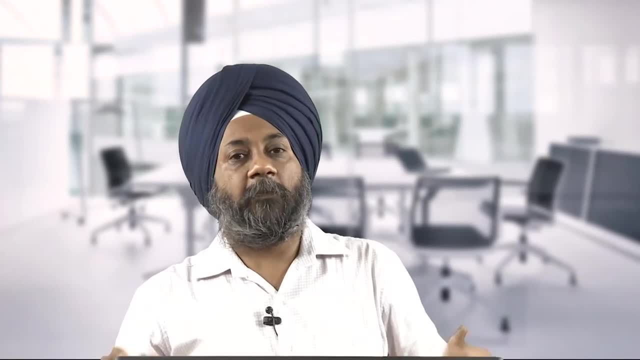 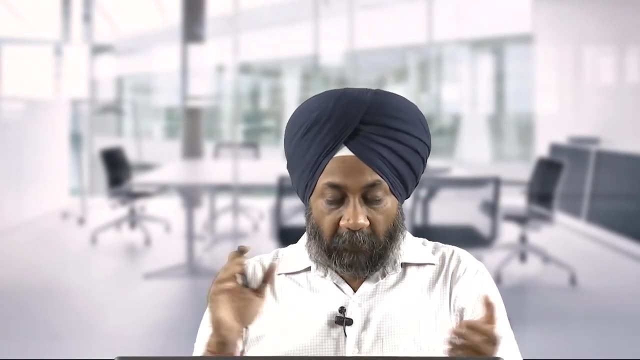 So you will increase the surface roughness by rubbing the sandpaper on the surface. So first and foremost, we have to prepare the surface. So this is the first step We have to. second is apply the adhesive. third is apply the pressure, or sometimes the heat. 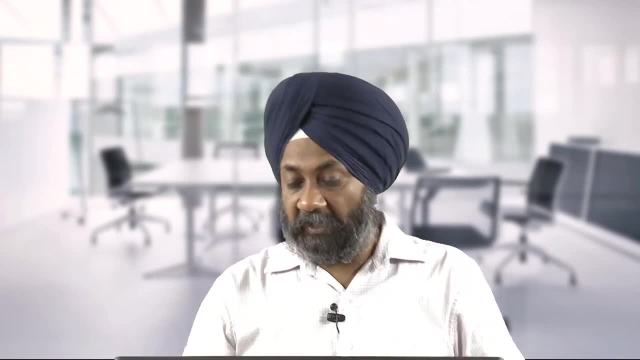 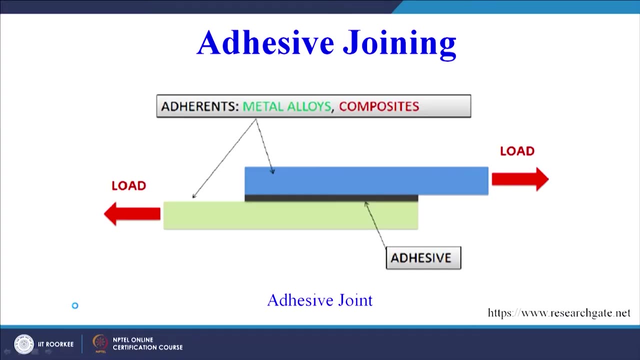 may be supplied and curing of the joint will take place and then the joint will be formed. So these are the 3 steps. again, this is explained here. we can use metal alloys, also that drains, composites can be used. this is the load that is being applied. this is the joint, the black. 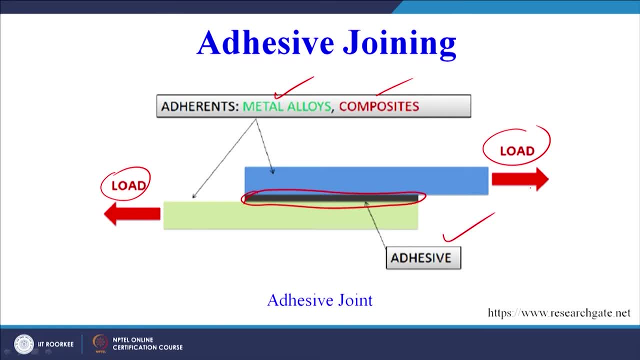 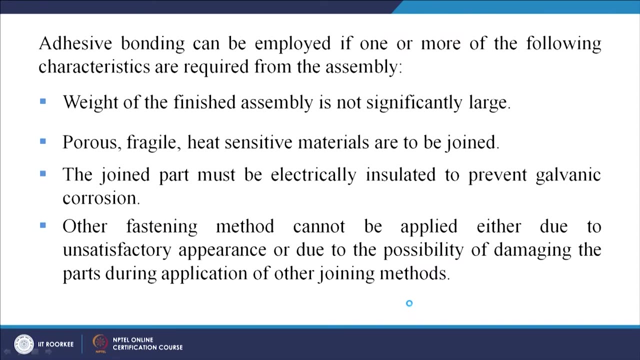 portion and this is the adhesive which has been used. this is the adhesive joint. So we can see very easy process, very simple process. no expertise is required. maybe little bit of training can help you to make the adhesive joints. Now, adhesive joining can be employed if one or more of the following characteristics are: 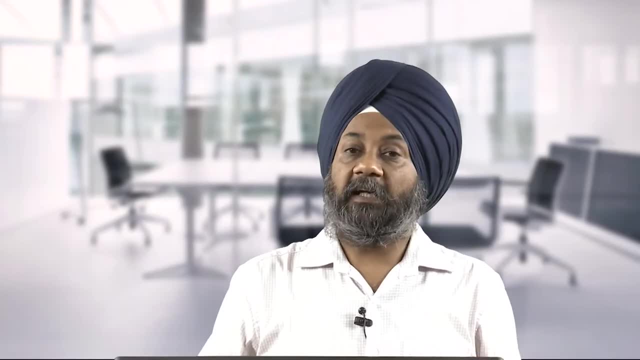 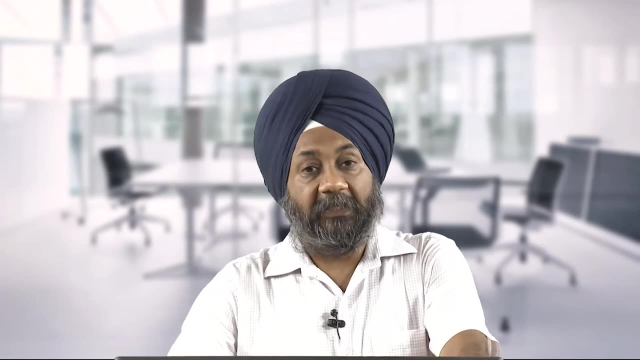 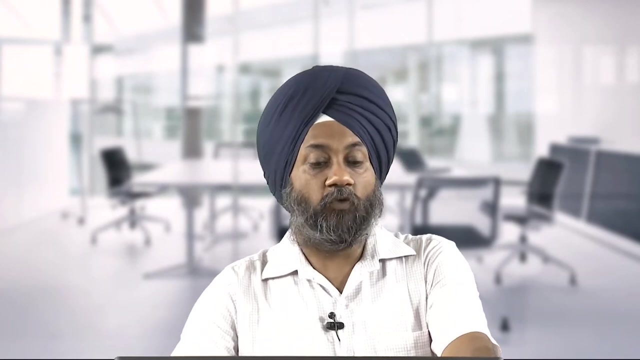 required from the assembly. Now, when we have done assembly, we are going to do the assembly of 3 or 4 different parts together. What are the essential characteristics that are there in the assembly? That is the assembly? That is the assembly That will ensure that we can make use of adhesive joining there. 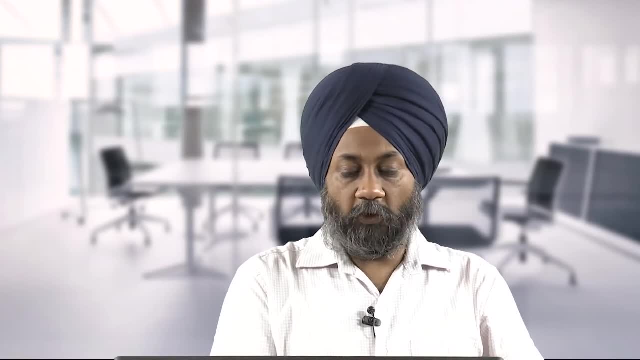 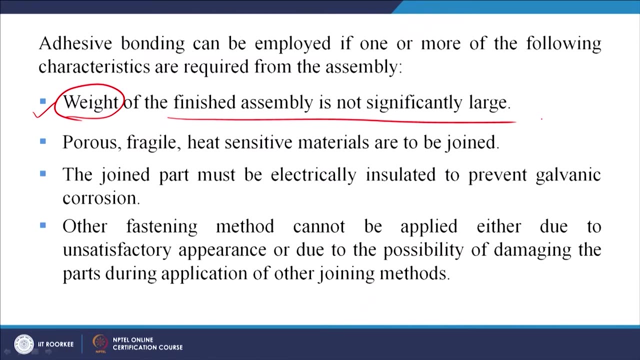 First characteristics is: weight of the finished assembly is not significantly large. So if the weight of the assembly is less, we can easily go for the adhesive joining approach or adhesive bonding technique. Then if the parts are porous or they are fragile or they are sensitive to heat, they are to 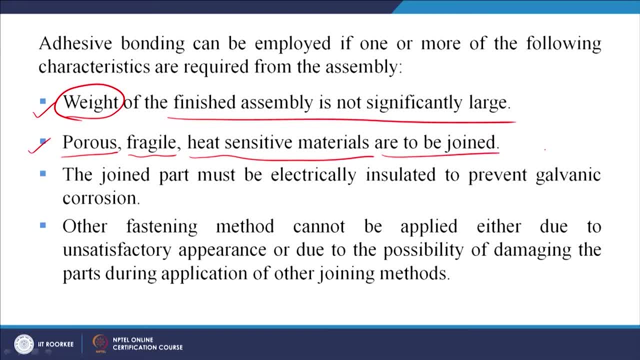 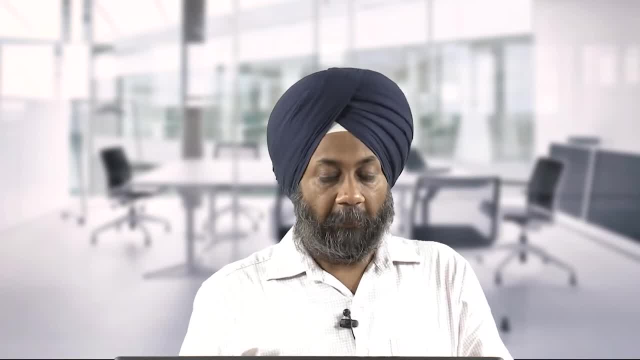 be high heat sensitive materials are to be joined. So when these type of material, which are porous, fragile, heat sensitive, in that case also we can go for adhesive joining. The joined part must be electrically insulated to prevent the galvanic corrosion. 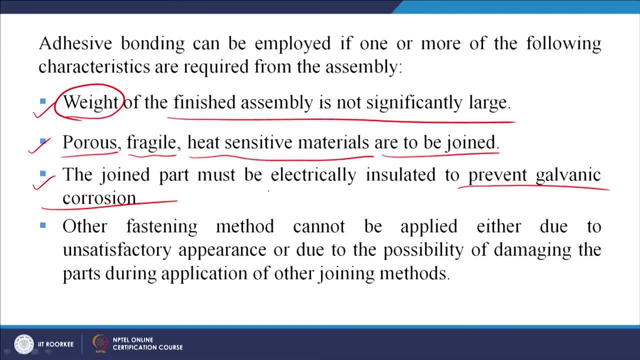 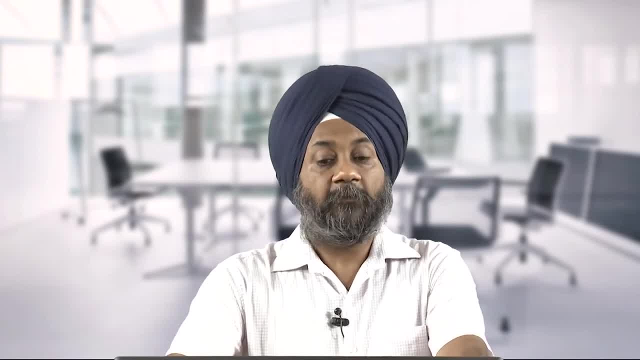 So when the galvanic corrosion has to be prevented or avoided and the joined parts has to be electrically insulated, in that case also adhesive joining is used. Other fastening method cannot be applied. Other fastening method cannot be applied Either due to unsatisfactory effect. 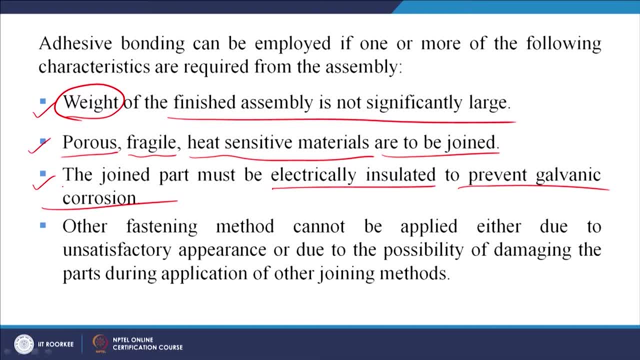 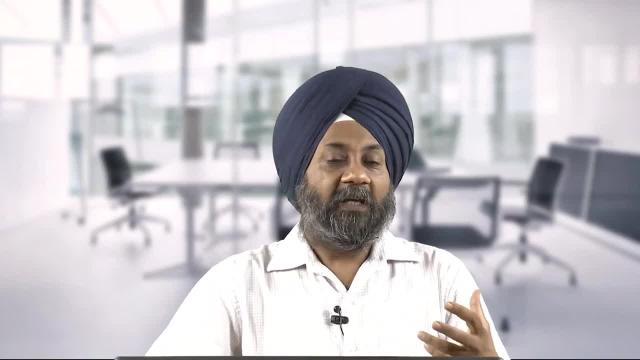 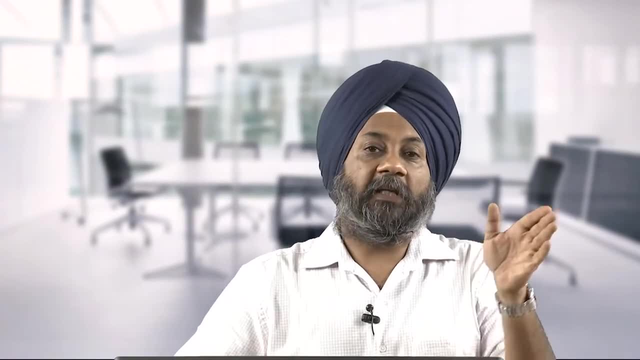 Either due to unsatisfactory appearance or due to the possibility of damaging the parts during the application of other joining method. So if you are applying a joining method, maybe you are trying to make a hole and then you will use a fastener to make the assembly and in that hole- making operation- you are damaging. 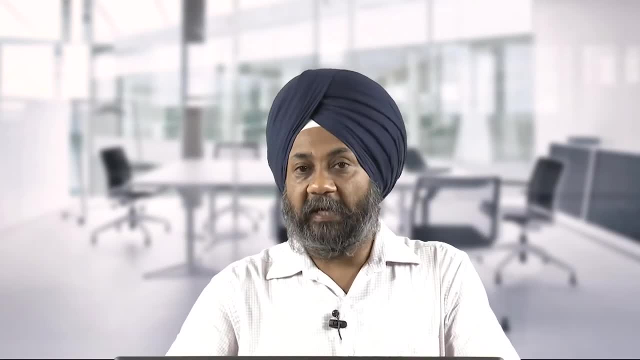 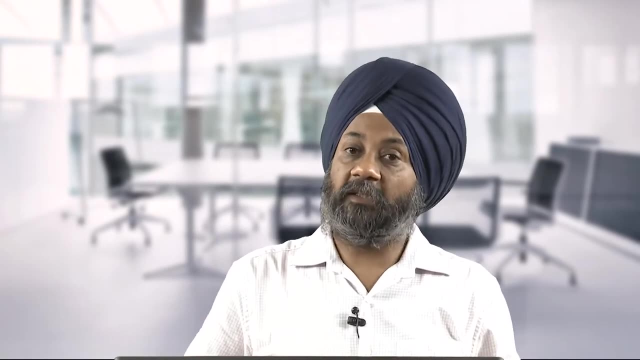 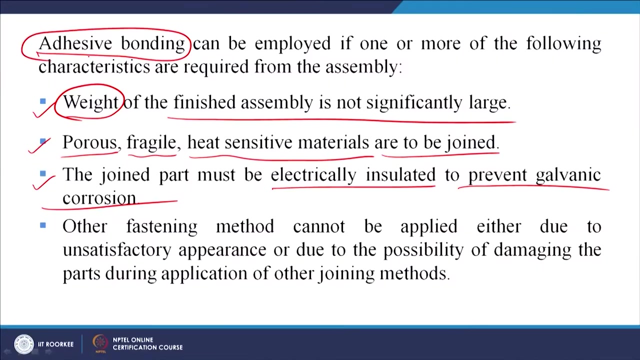 the part. in that case you may not be able to use the mechanical fastening technique, So you will very easily go for adhesive joining technique there. The other joining methods are not possible, So there also you can apply the adhesive bonding or adhesive joining technique. 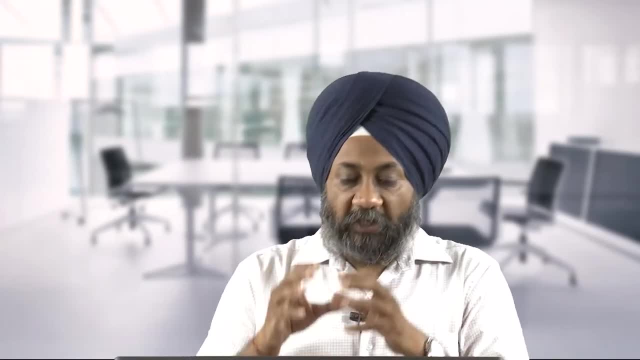 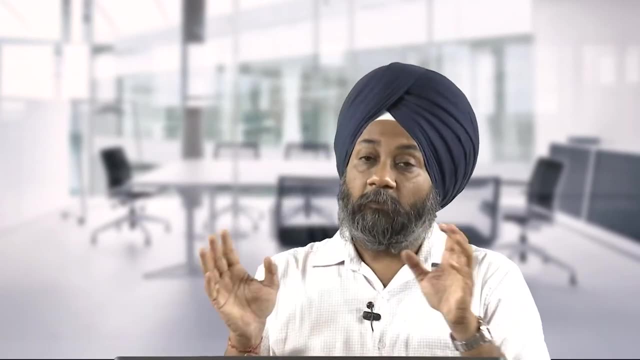 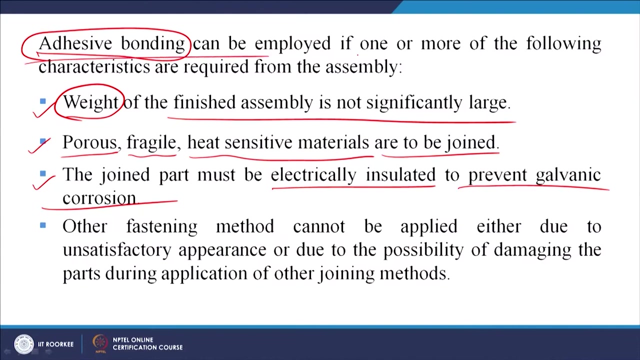 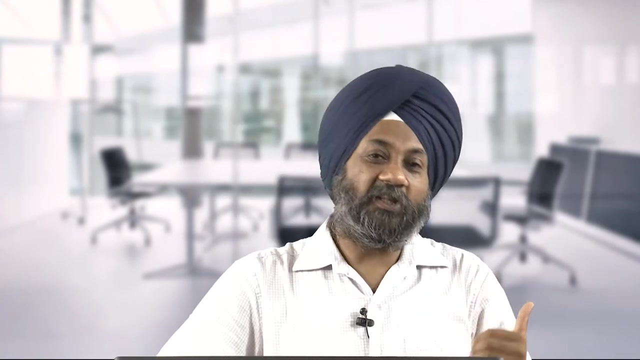 So, in summary, lightweight, porous, fragile, heat sensitive materials, as well as where electrical insulation is required, wherever the galvanic corrosion is an issue. in all those cases, you can very easily use the adhesive bonding technique. So, as a product designer, now We can keep in mind all these points that in these cases, we must suggest, we must design. 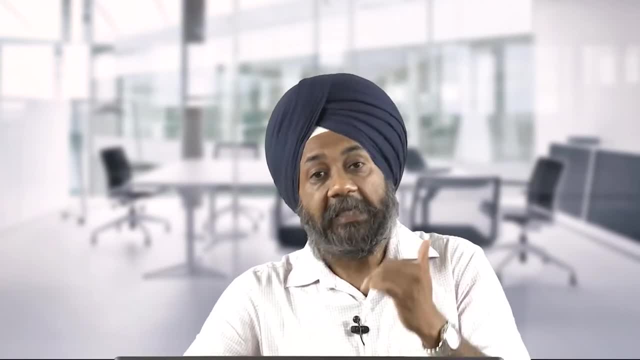 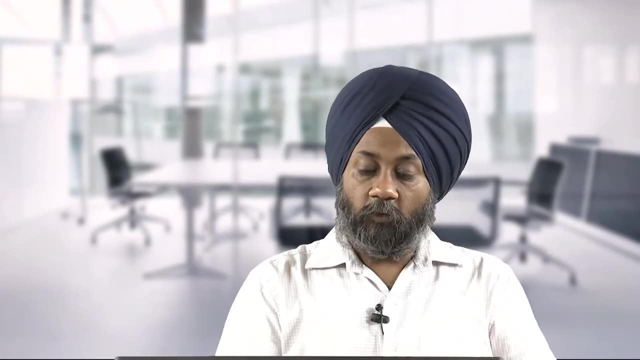 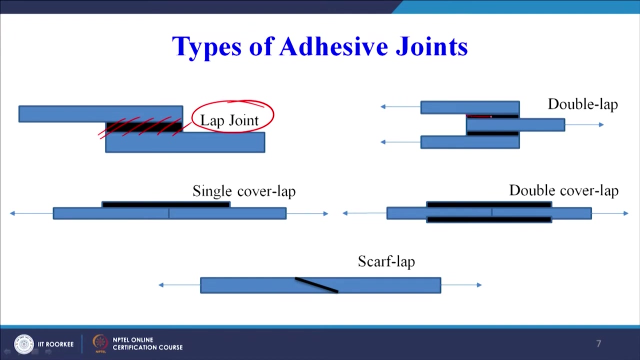 our part in such a way that these parts can be easily joined using the adhesive bonding technique. Now, different types of adhesive joints can be there. one is a lap joint, this is a joint area or the joint interface. Then double lap, this is one. adhesive bonding, this is second. 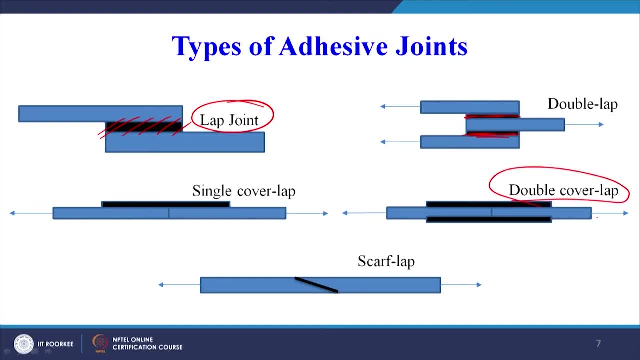 Then double cover, lap joint. we can see this is double cover. is there? this is the overlap area here. Then the scarf. we can see this is a scarf joint. this is single cover. lap cover lap is on one side only here it is on 2 side. 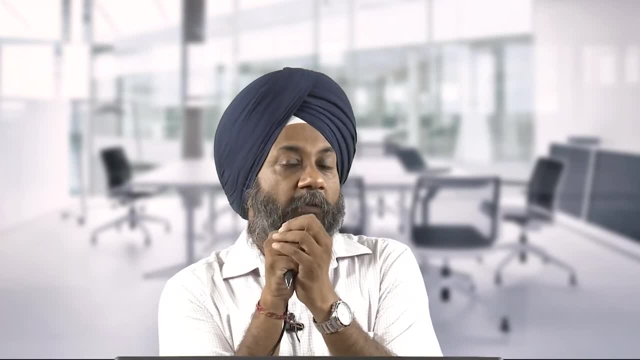 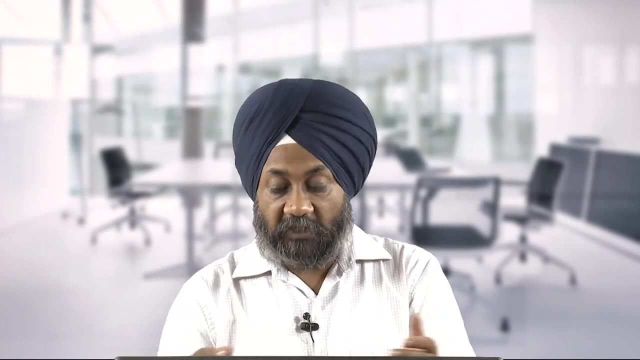 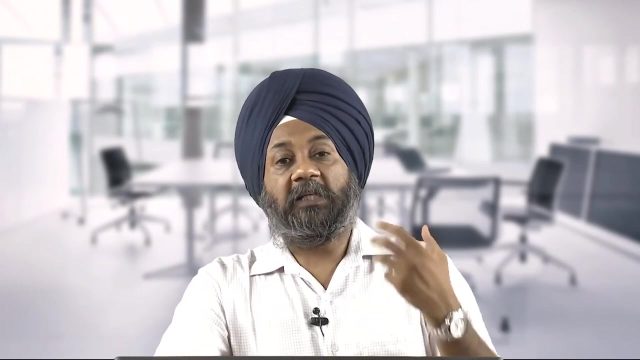 So you can decide your product, that what type of joint will be able to help you to join the 2 parts together. So different joint configurations you can select. there is a wide variety, even you can design your own. So different joint configuration. only thing is, the 3 steps will remain same. that is preparation. 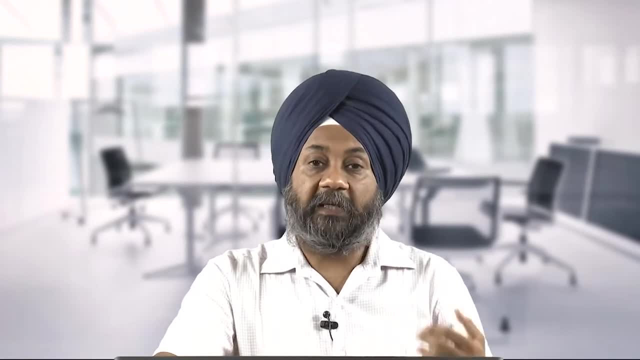 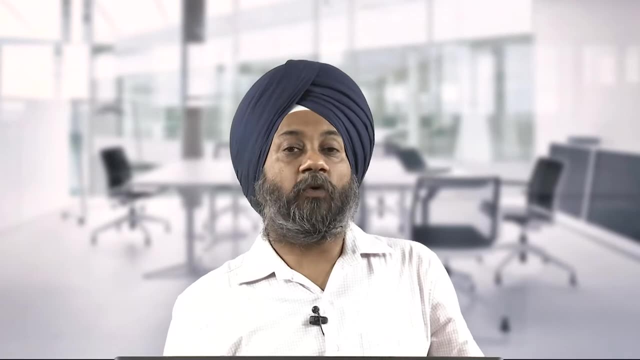 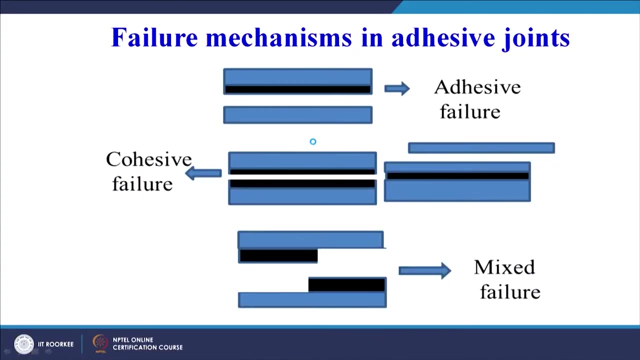 of the surface, application of the adhesive and finally, curing of the adhesive under heat and pressure. So these 3 steps remain same, the joint configuration you can design as per your requirement. Now these are the failure mechanisms. slightly, we are going into the depth now. these can: 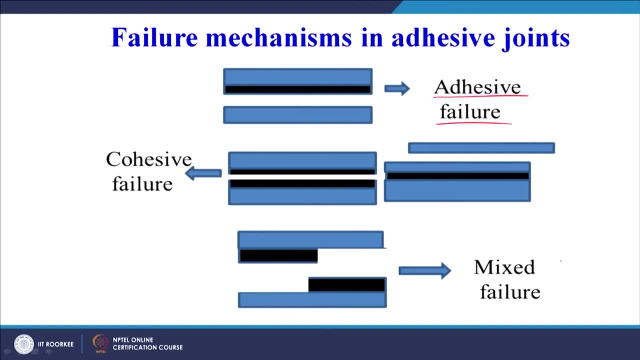 be adhesive can fail adhesive failure. there can be mixed failure. this can get debonded from here and the adhesive has also failed from here. then there is a cohesive failure here. So different types of failure may take place when the product is loaded under the different 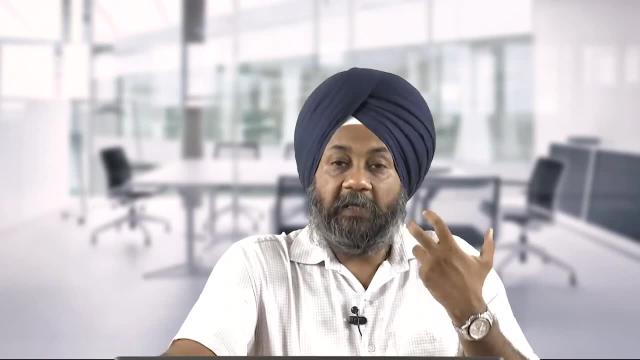 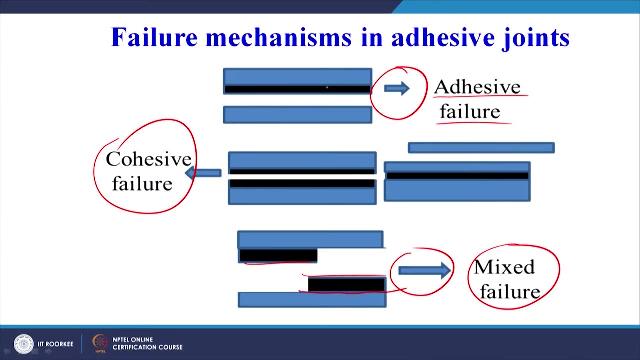 types of loading environments. It can be compressive load, it can be tensile load. here we are showing tensile load only, but it can be under compression and the shear. under different types of loading environments the failure might be different Depending upon the kind of body. 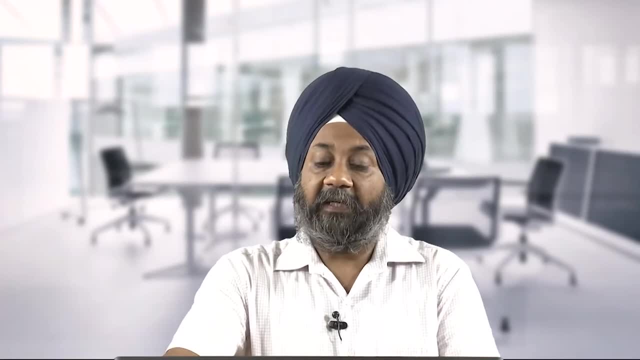 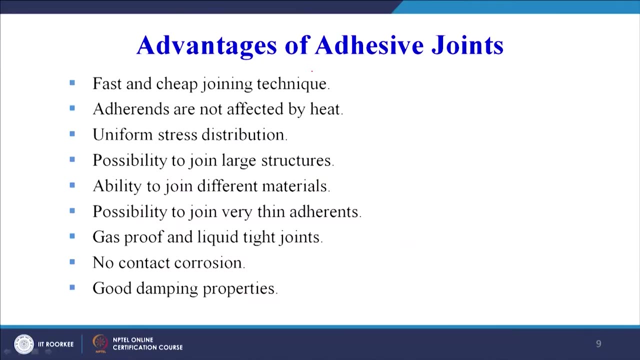 The bonding that has been developed between the 2 adherents. Now what are the advantages of the adhesive joint? fast and cheap? I will just read: if you have understood the adhesive joining, it will be easier to understand fast and cheap joining technique. adherents are not affected by heat. maybe adherents are not effective. 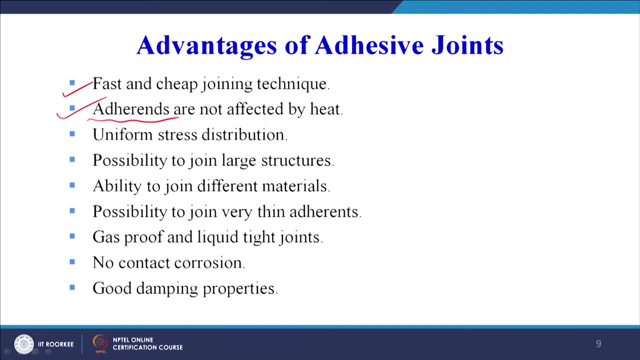 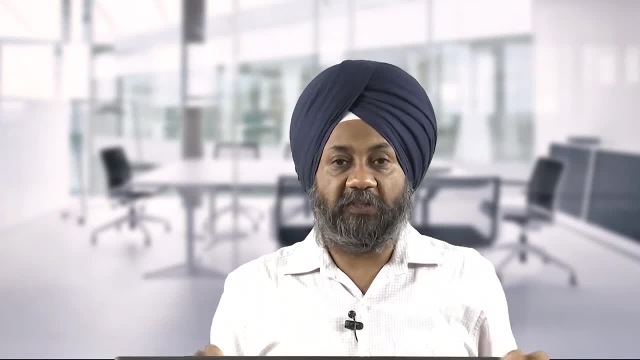 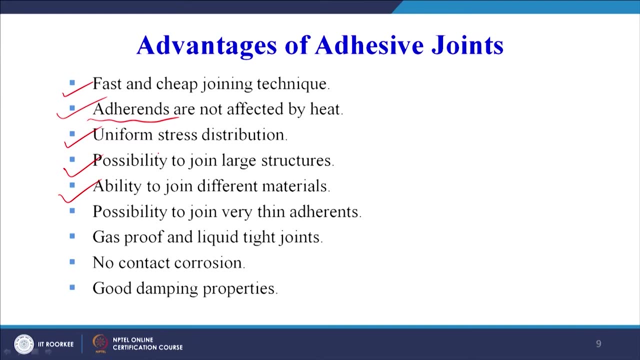 But if lot of heat is there, the adhesive may get affected by the heat. if in service you find lot of heat, uniform stress distribution. no stress concentration is there Uniformly. the stress is distributed over the whole adhesive area. Possibility to join large structures. ability to join different materials: different materials. 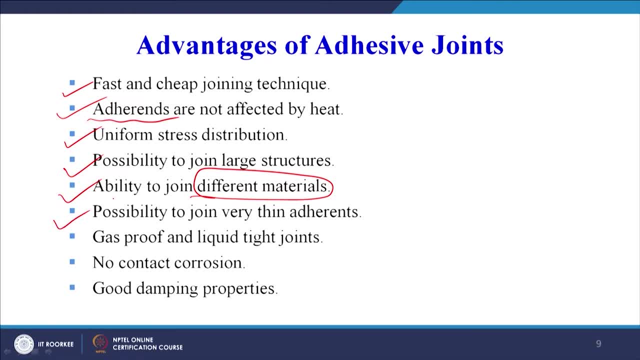 as we have seen, the adherents can be of different material. Possibility to join very thin adherents also, which is otherwise very difficult. gas proof and liquid tight joints can be made. no contact corrosion- galvanic corrosion is also avoided. good damping properties. So 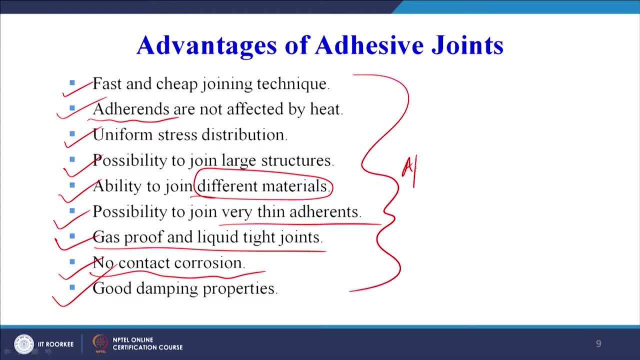 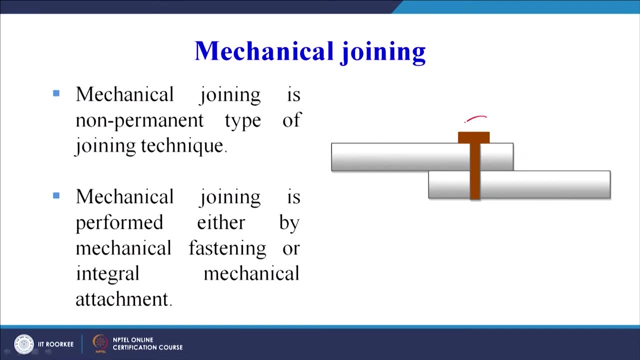 You can see a long list of applications where the adhesive joints can be easily used. So these are the areas where a product designer can think of using the adhesive bonding or joining techniques. Now, coming on to the mechanical joining, all of us have seen number of application areas. 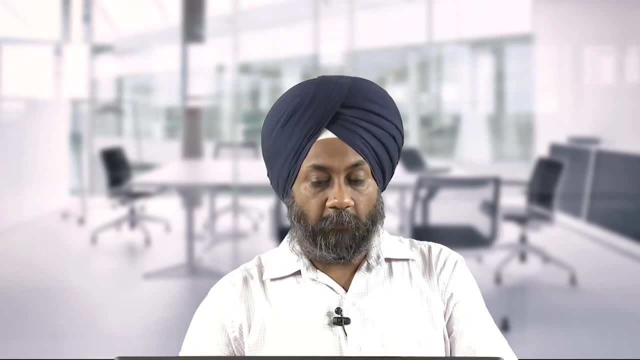 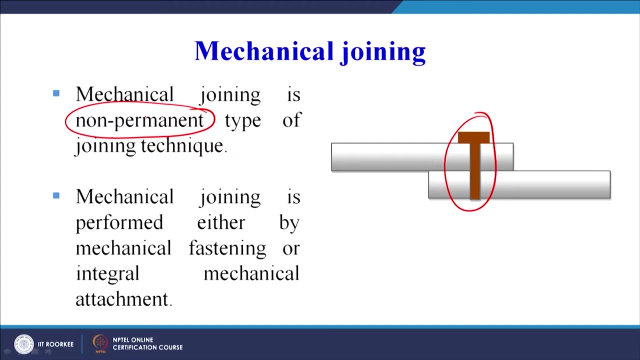 of the mechanical joints. So mechanical joining is a non-permanent. why it is non-permanent? because we can always unbolt the joints. So mechanical joining is a non-permanent type of joining technique. mechanical joining is performed either by mechanical fastening or integral mechanical attachments. 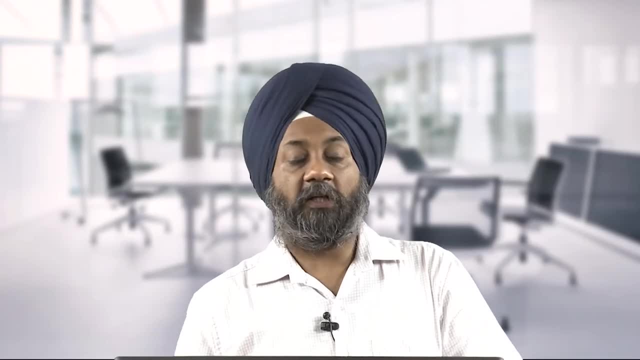 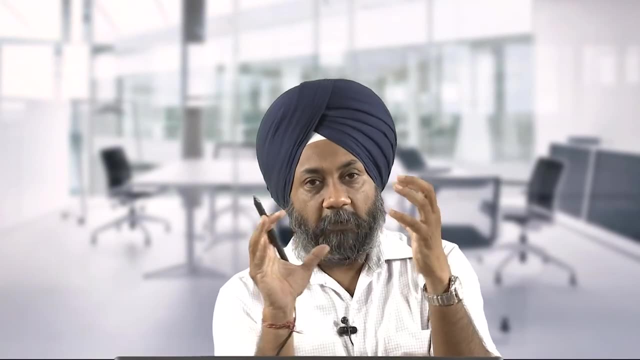 So you can do maybe the fastening using a fastener, or it can be integral permanent attachment of mechanical type So you can permanently use a mechanical fastener in your assembly. So fasteners, we can see we got 2 types: rivets as well as your screw fasteners. 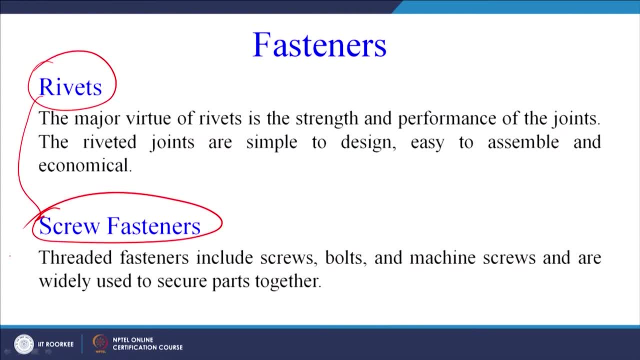 So 5 types of fasteners. So fastener, bolt fastener or screw fastener. So 5 types of fasteners. So what are rivets? the major virtue of rivets is the strength and performance of the joints. the riveted joints are simple to design, easy to assemble and economical. 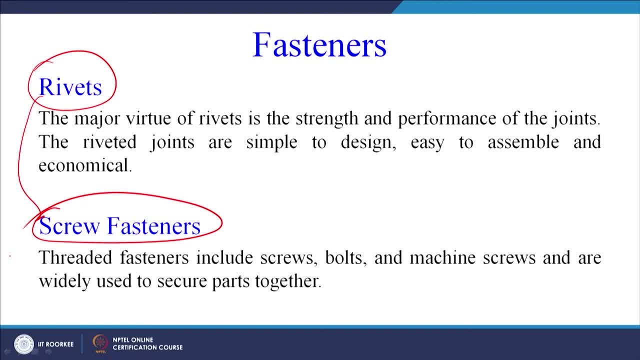 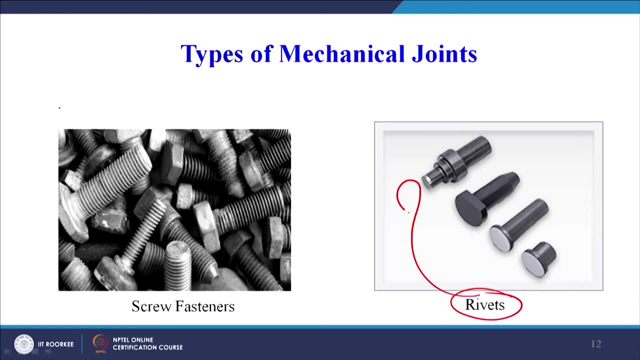 Screw fasteners. threaded fasteners include screws, bolts and machine screws and are widely used to secure the parts together. so 2 types of fasteners are used: rivets and the screw fasteners. Now these are the types of mechanical joints. you can see the rivets here, different types. 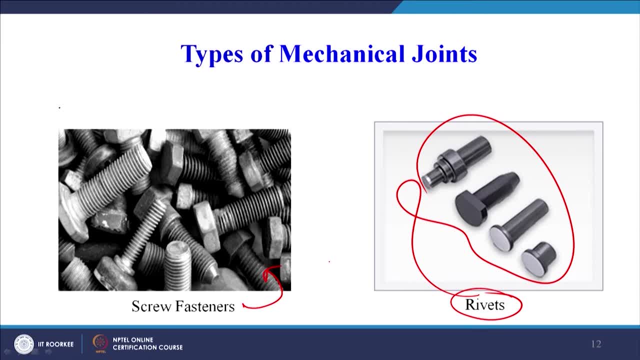 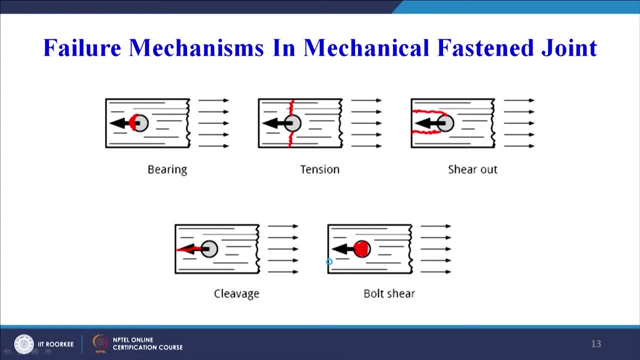 of rivets are there and these are the screw fasteners or the threaded fasteners. Now failure mechanisms in mechanical fastened joints we can see here we can have a bearing type of failure under tension. this is the type of failure which may take place: shearing. 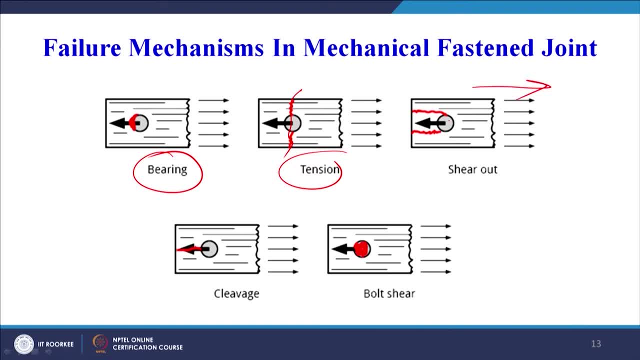 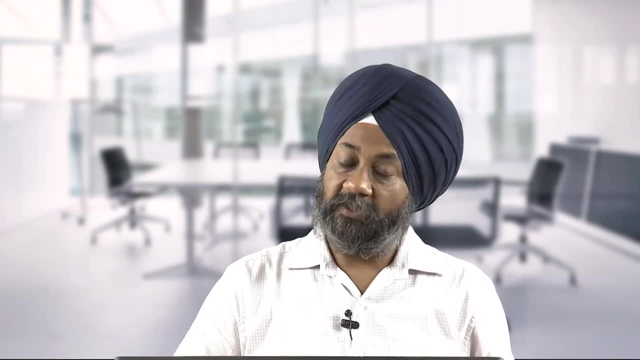 out. we are applying the load in this direction and this may shear out in this direction. Then cleavage can be formed. it is shown here. it is a bolt. shear can also take place. the bolt may also. The work piece may fail or the bolt may also fail in some cases, depending upon the type. 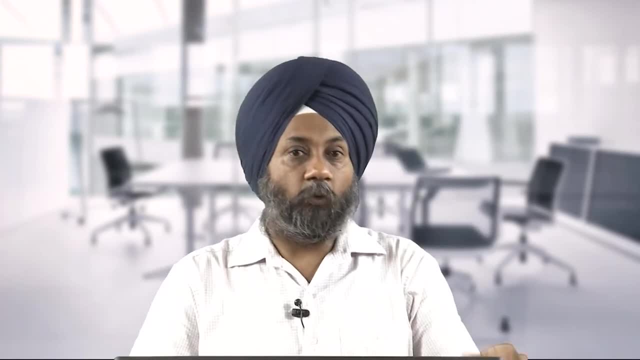 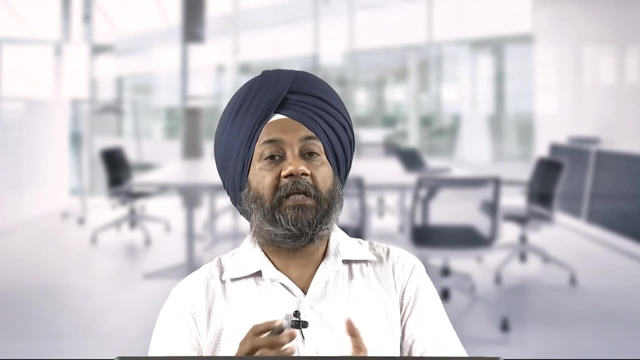 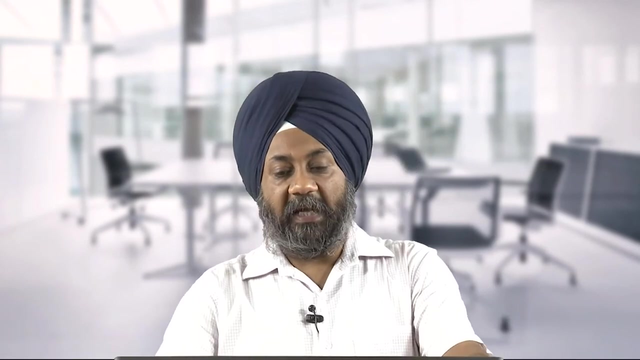 of loading environment, depending upon the material of the bolt that we have selected, depending upon the material of the adherence that we are using, different failure mechanisms may take place during the loading of the mechanically fastened joints. Now, what are the advantages of mechanical joints? these allows intentional disassembly. 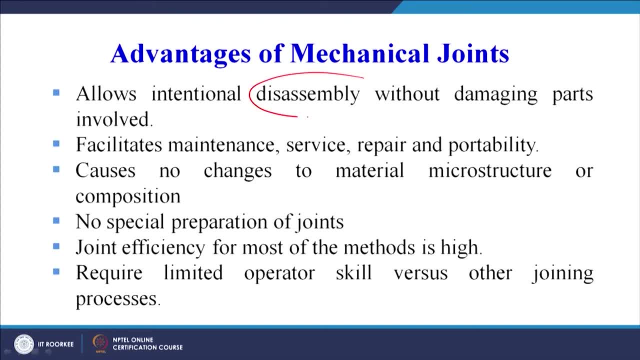 without damaging the parts involved. This is As we have seen. it is not a permanent joining technique, so we can disassemble the structures also where mechanical joints or mechanical fasteners are used, facilitates maintenance, service, repair and portability, which is a direct reflection of the first point. 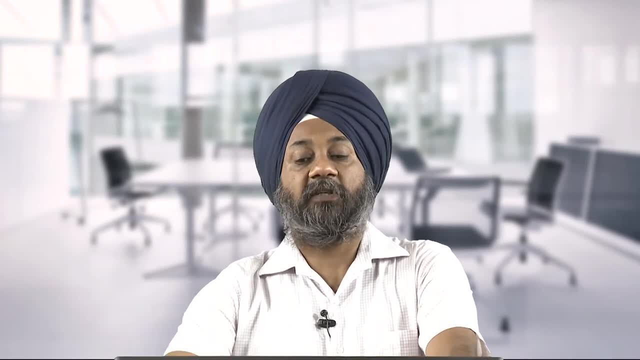 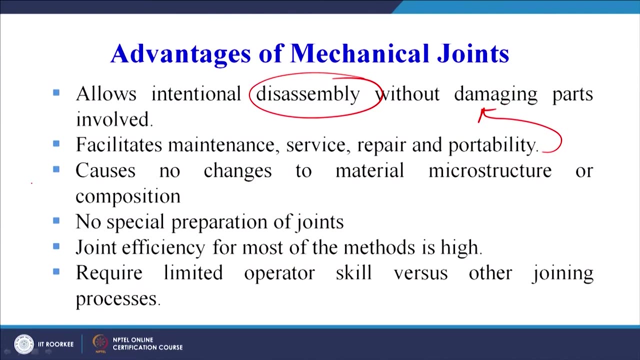 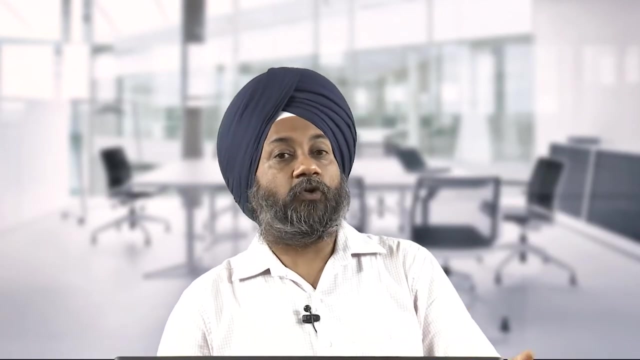 If you can disassemble your structure, you can easily do maintenance, service, repair and portability. This causes no change to the material, microstructure or composition which is in contrast to, which is in contrast to the adhesive joining technique, as well as the welding, where the microstructure 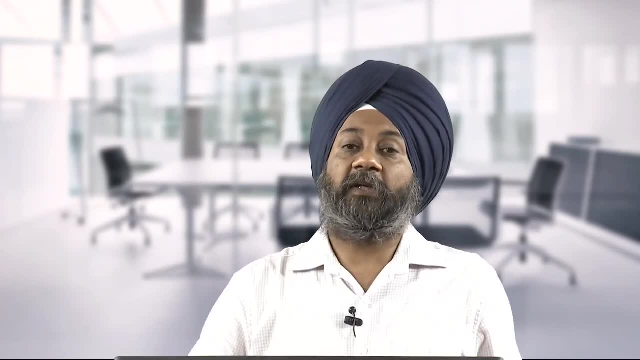 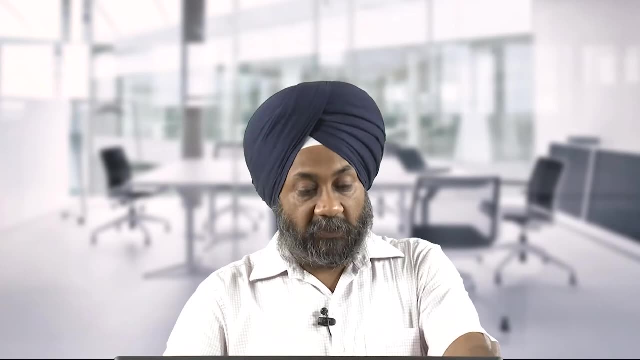 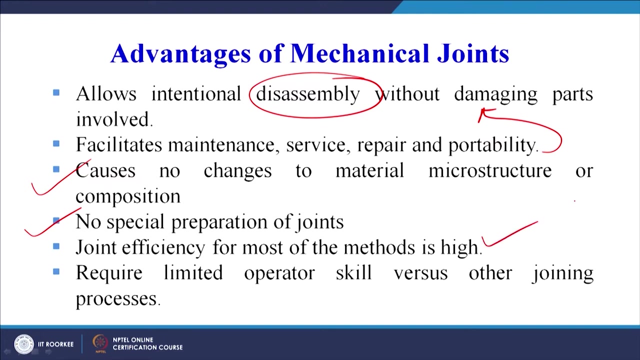 may take place In adhesive joining also. we do the surface preparation, so the surface morphology is affected in case of adhesive joining. but here no such problem is there. No special preparation of joints is required. joint efficiency for most of the methods is high. 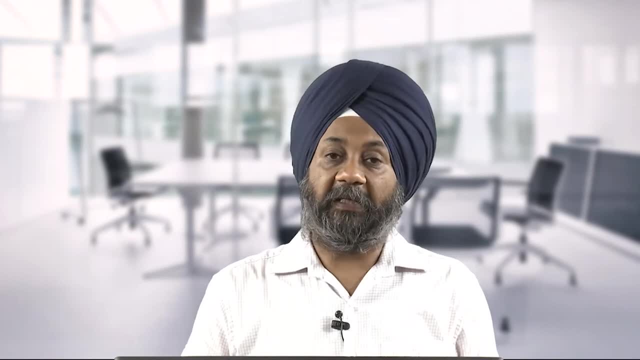 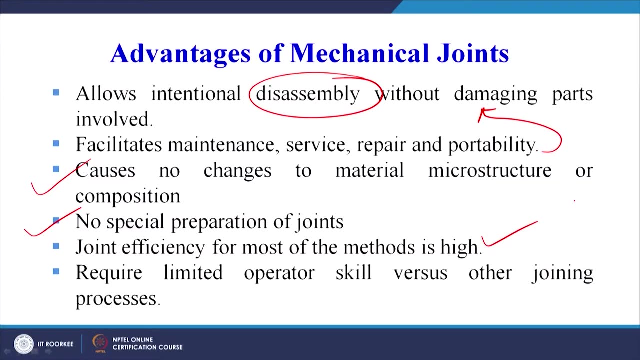 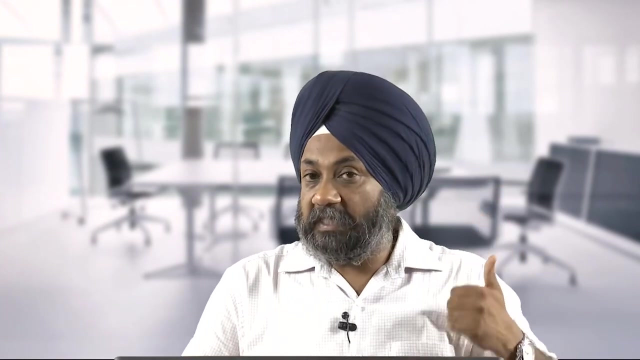 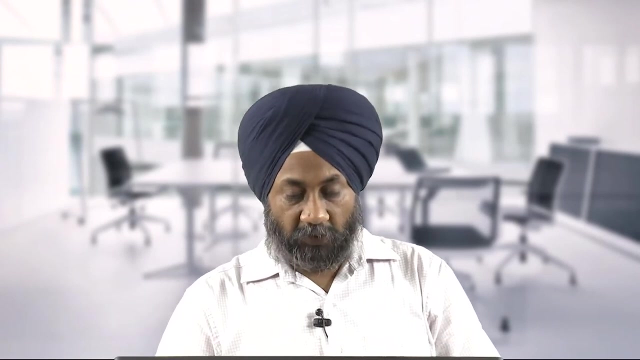 So as compared to adhesive joining the joint efficiency is better. in case of mechanically fastened joint require limited operator skill versus other joining processes. So for adhesive joining also minimum skill set is required, whereas in adhesive joining minimum skill set is required. In mechanical fastening it is still easier, easily a person can do the assembly operations. 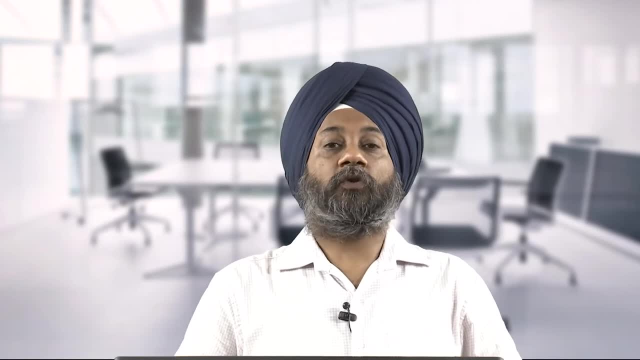 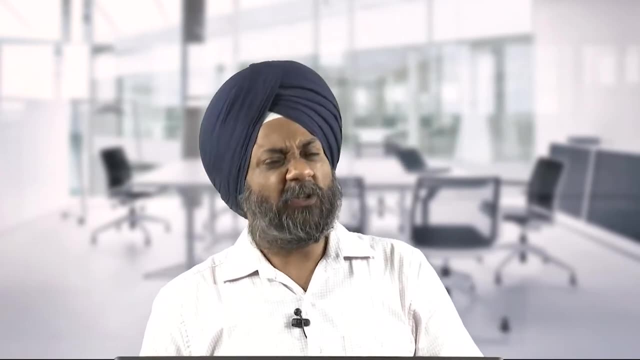 most of the time, it is done manually. Now, coming on to the last process: we are also running out of time, so welding is a very, very important process And it has been dealt in In much more detail. there are courses available under MOOC scheme focusing on welding. 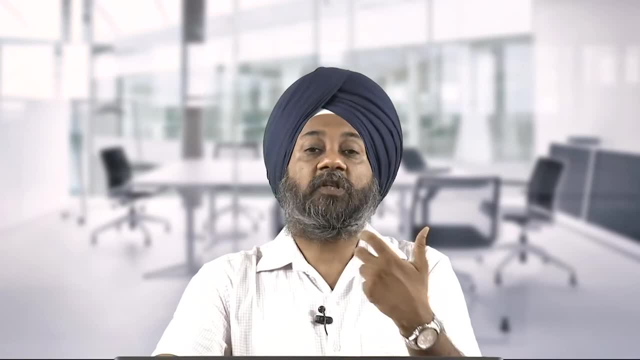 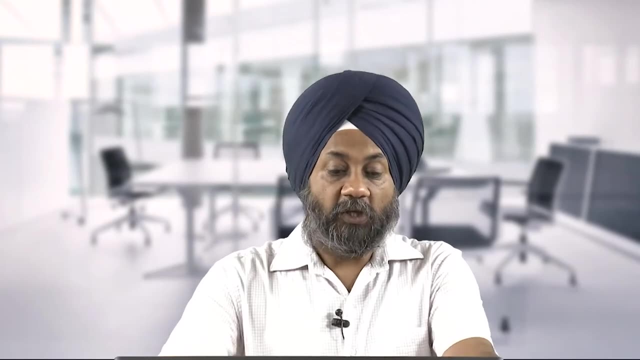 But we will just try to highlight to our learners what is welding, so that when you design a product you understand the basic intricacies involved in the welding process. So welding is a process in which material of a similar type or a class are brought together. 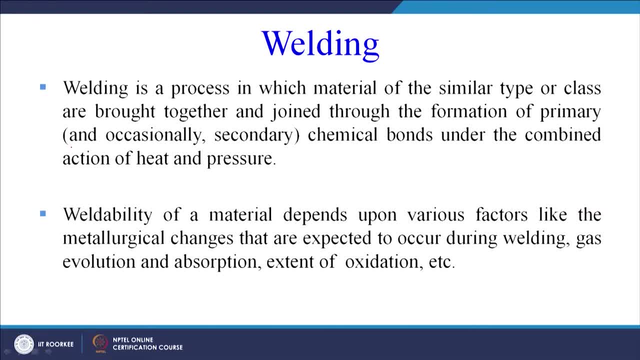 and joined through the formation of primary and occasionally secondary chemical bonds under the combined action of heat and pressure. Thank you, So one thing I would like to suggest here. in this definition so little change: welding is the process in which material of similar type or class. 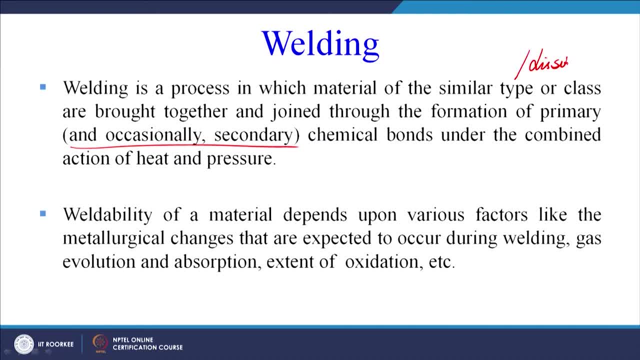 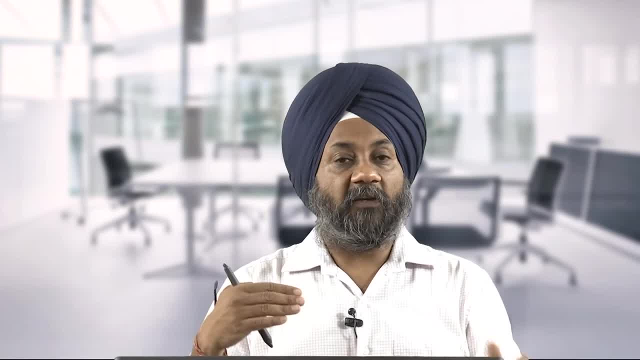 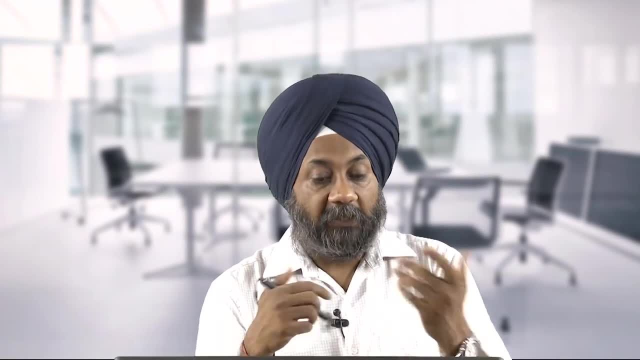 So these days we have processes where we can use dissimilar materials also. So we have a welding technique, maybe a advanced welding technique, where dissimilar materials can also be joined. so we have to join the 2 materials together, either by formation of primary or secondary. 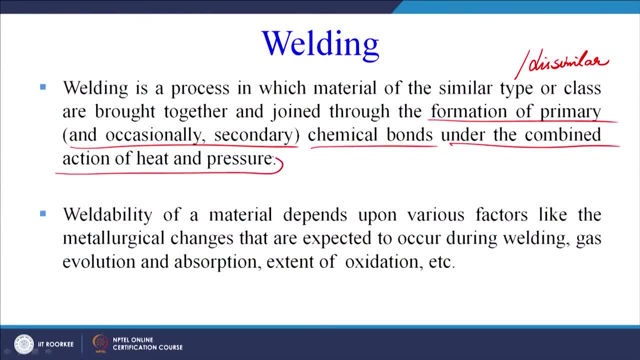 So these are the 2 important inputs, heat, and the other input is the pressure. So we have to join the 2 pieces together, forming a joint here by the application of heat and pressure. Weldability of a material depends upon various factors, like the metallurgical changes that 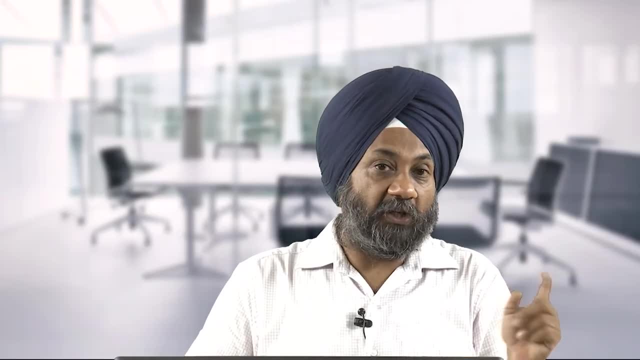 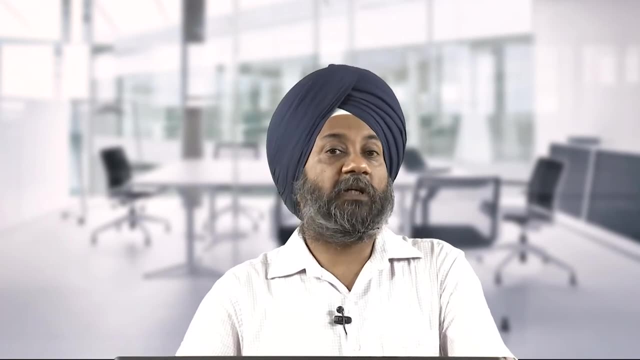 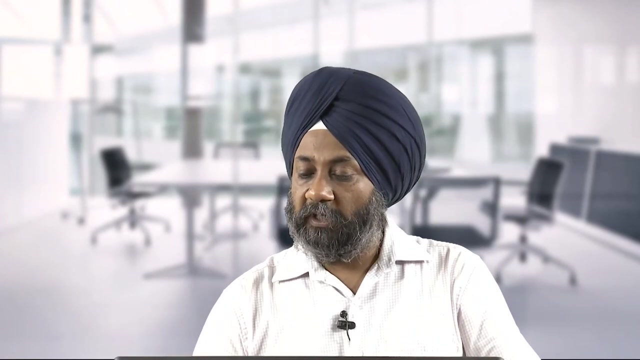 are expected to occur. We have seen that in mechanical fastening no changes occur at the metallurgical level. But in welding metallurgical changes of the microstructure of the 2 metals which you are joining together is definitely going to change, Because here one of the inputs is heat. so when you heat the material above its melting, 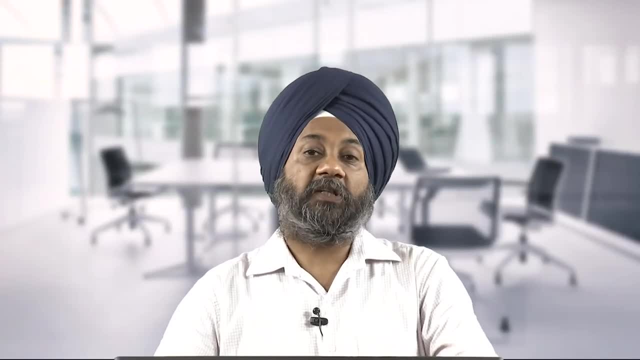 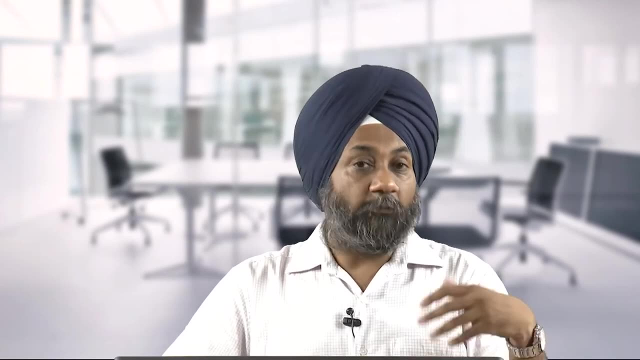 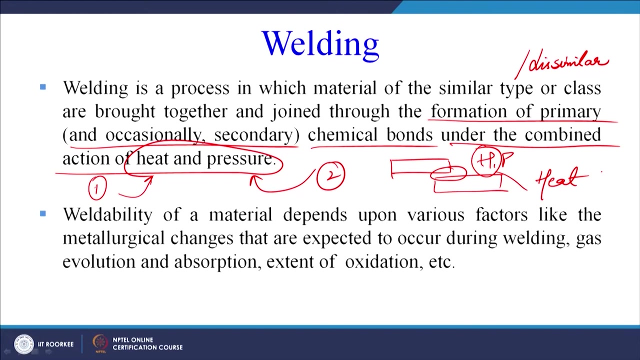 point and then you allow it to solidify. Certainly, certain metallurgical changes are going to happen. so the metallurgical changes that are expected to occur During welding, During welding, will definitely govern the weldability of the material: gas evolution and absorption, extent of oxidation. 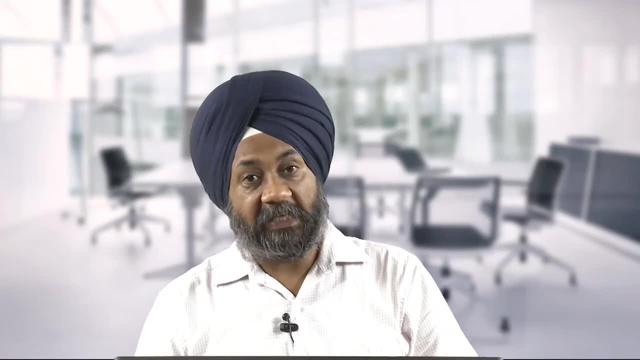 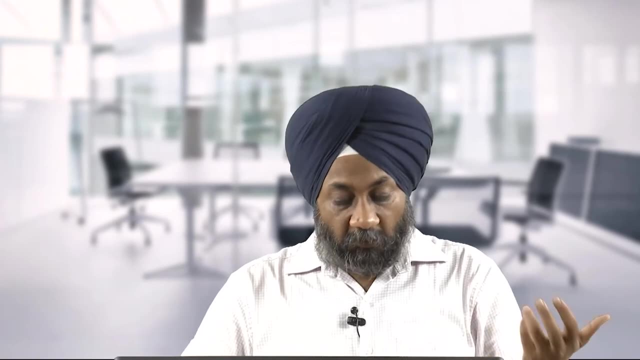 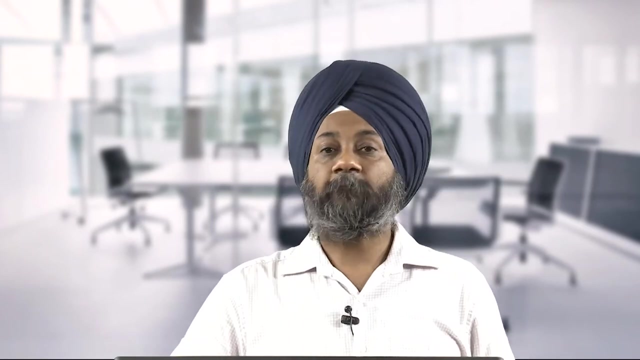 So usually we say aluminium oxidizes very easily. So maybe the materials that we are going to weld it, the characteristics like oxidation, evolution and absorption of gases, metallurgical changes expected- are going to affect the weldability of any material. So when we are selecting a material for our product, 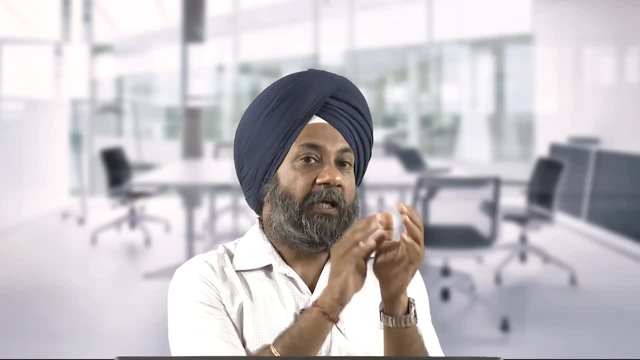 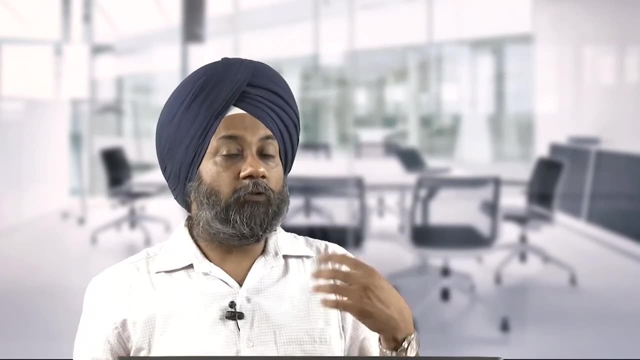 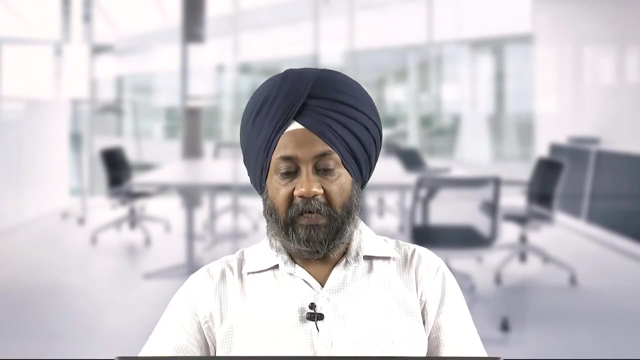 And we feel that later on it has to be welded to another part in order to get our product. In that case we must be very, very careful and study that what kind of metallurgical changes can happen during the welding process which may affect the performance of our product? 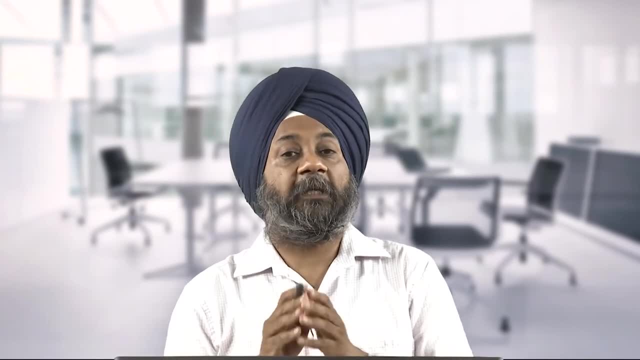 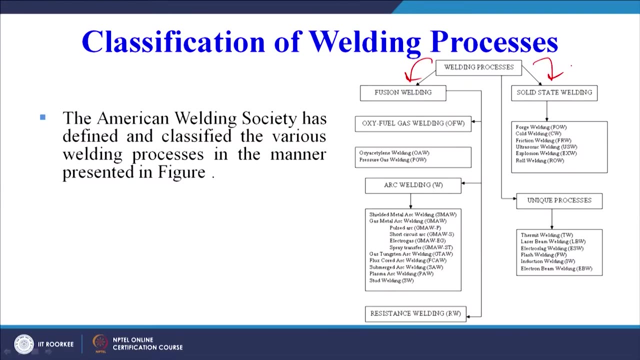 And welding is a very, very diverse field, a very, very exhaustive field, and the welding processes are basically, you can see, classified into 2 major categories. We will not go into the details. Okay, We will go into the detail of each one of these. 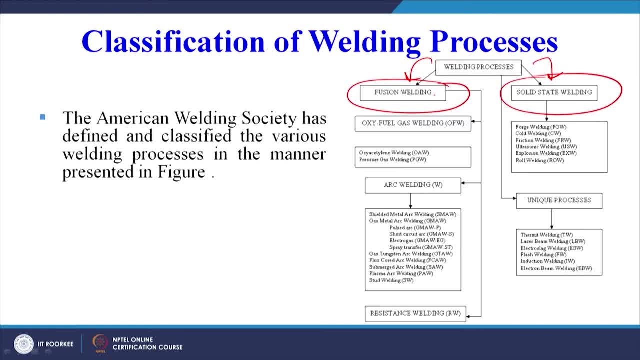 So the fusion welding and the solid state welding. So the American welding society has defined and classified the various welding processes in the manner presented in the figure. So this is the figure you can see. major classification is fusion welding and solid state welding. And in solid state welding we have an explosive welding technique: ultrasonic welding, friction. 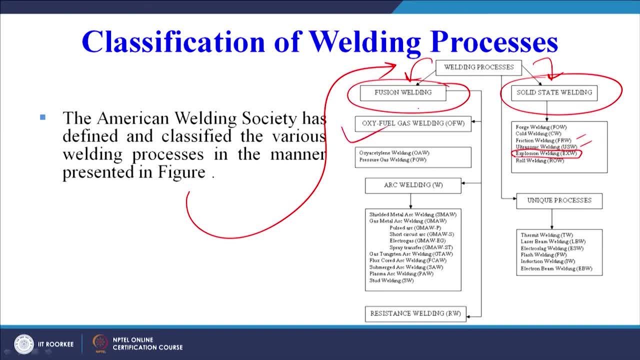 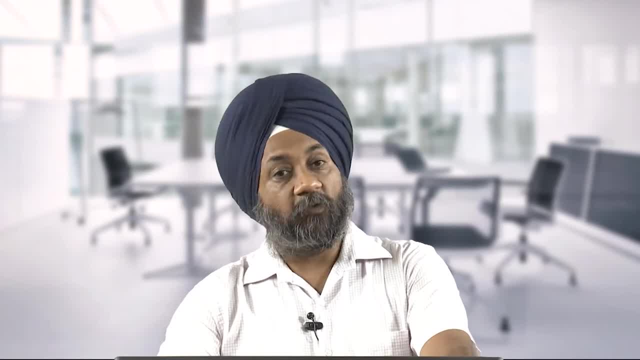 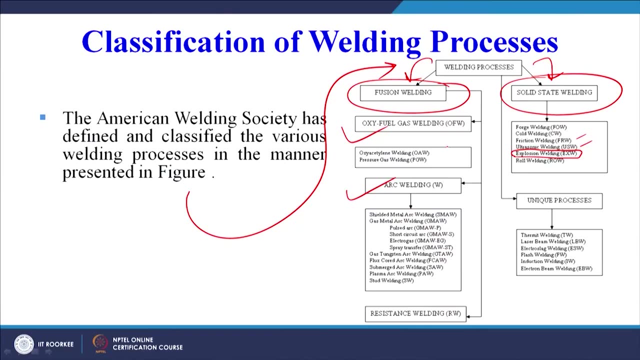 welding and in fusion welding. most common oxy acetylene gas welding And arc welding. so generally we use oxy fuel gas welding as well as arc welding. and arc welding has further classification like gas, tungsten arc welding, submerged arc welding, plasma arc welding, stud welding. 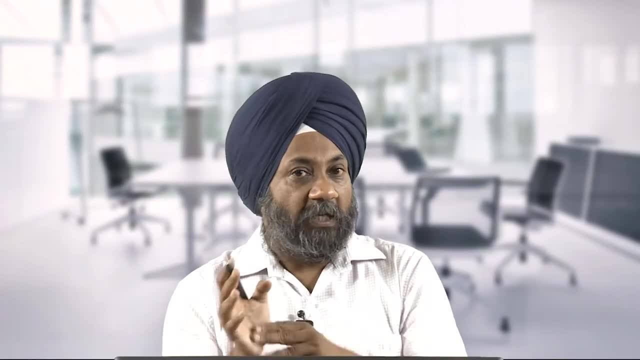 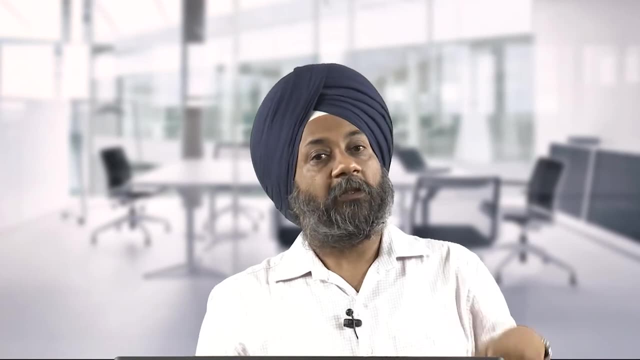 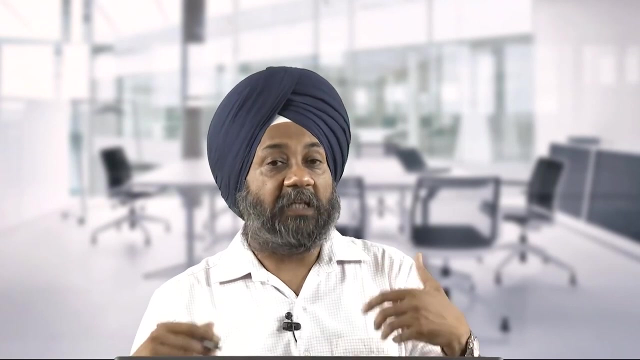 So we have different types of welding techniques available. so as a product designer, I must have a basic idea that when I am designing a product and it has to be welded during the product fabrication stage or during the product assembly, Okay, During the assembly stage I must take care of the choice of materials, the type of design. 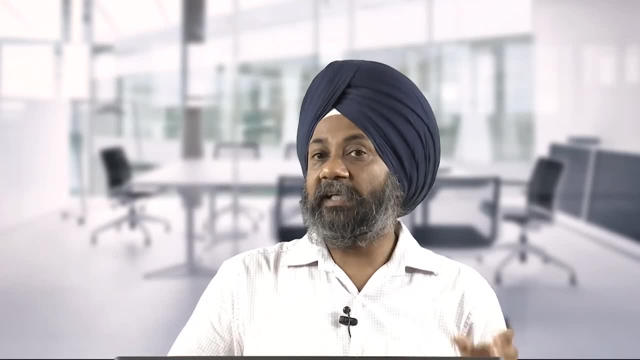 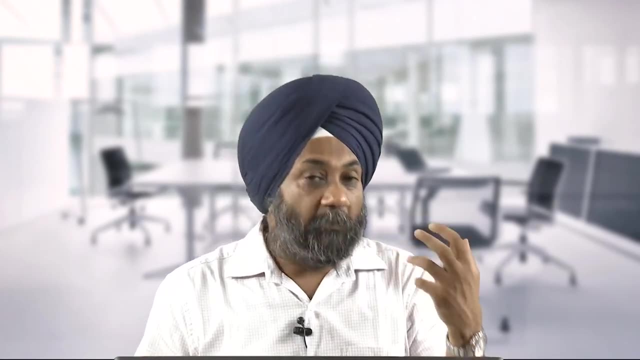 the geometrical features that I am putting in the product So that it is easier to assemble at a later stage. and for welding there is a wide variety of processes which are material specific, which are heat input specific, which are metallurgical changes specific. 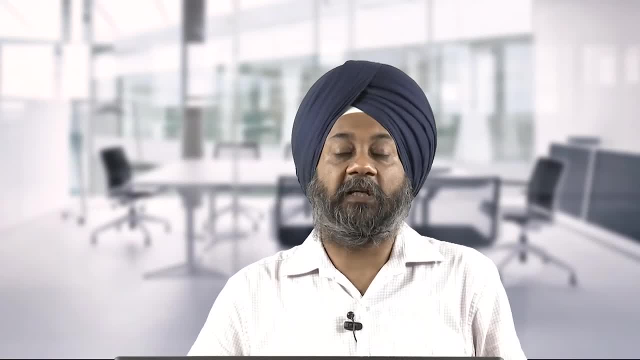 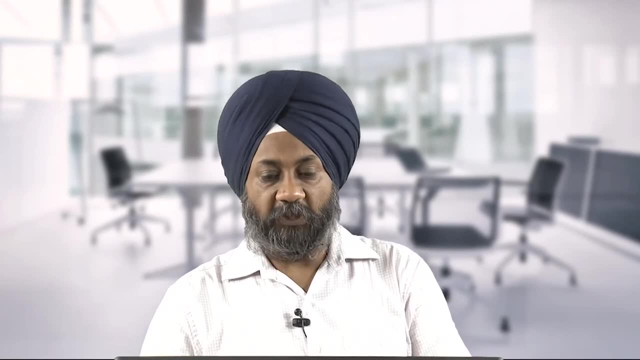 So, depending upon the various factors that influence the weldability of materials, we must choose the material as well as we must choose the appropriate order. Okay, So that is the specific process. So in fusion welding we will try to understand, because in the previous slide you have seen. 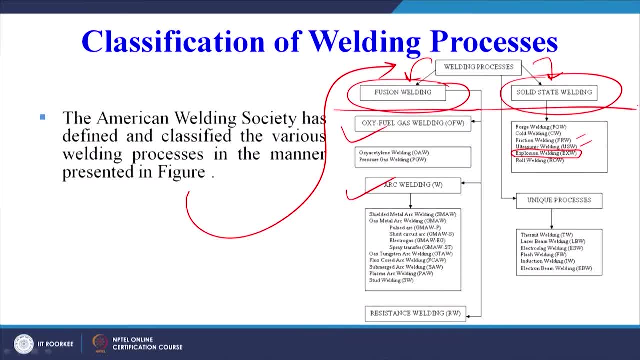 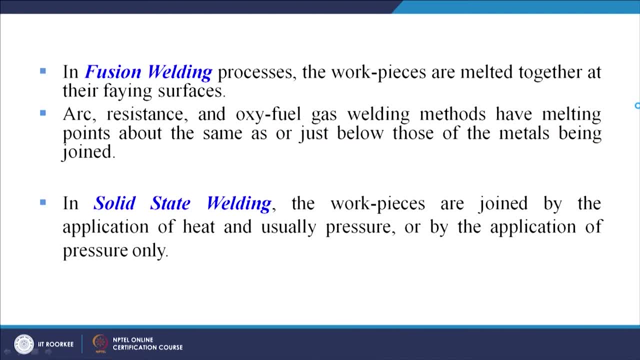 2 major categories are there: fusion welding and solid state welding, and then there are subcategories to these. So fusion welding: in fusion welding processes the work pieces are melted together at their faying surfaces. arc welding, resistance and oxy fuel gas welding methods are melting points. 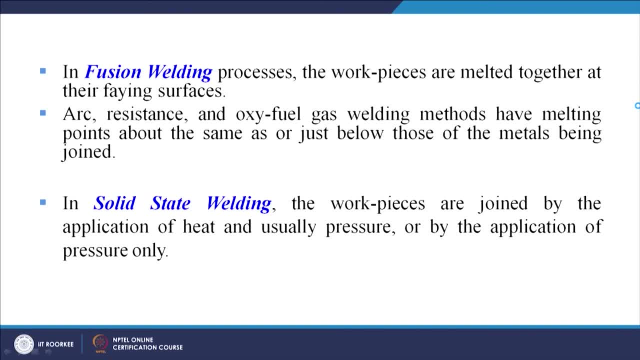 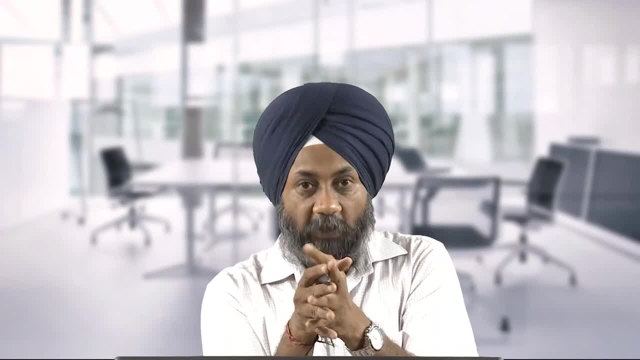 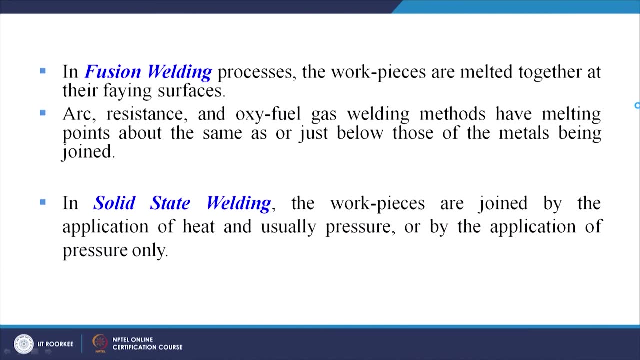 above, the same as or just below those of the metals being joined. Okay, So we will heat the metal, we will try to melt the metal and then fuse the metal together to form the joint. examples are given In solid state welding: the work pieces are joined by the application of heat and pressure. 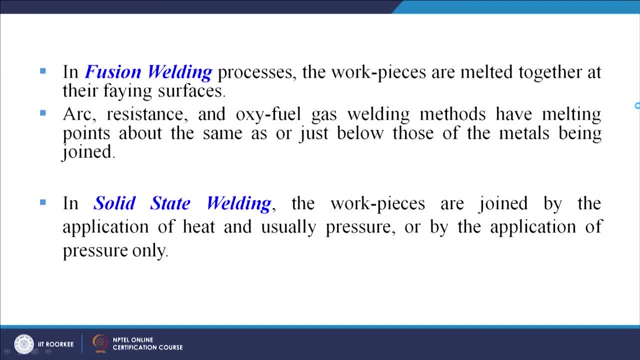 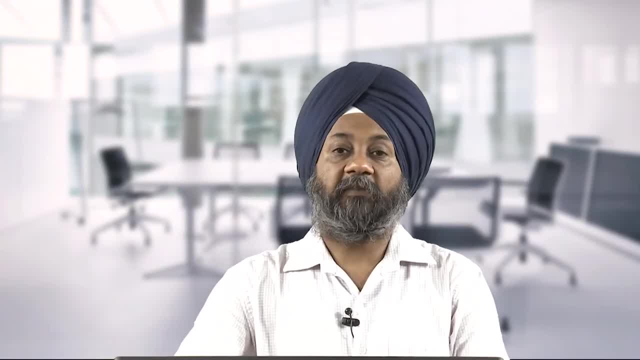 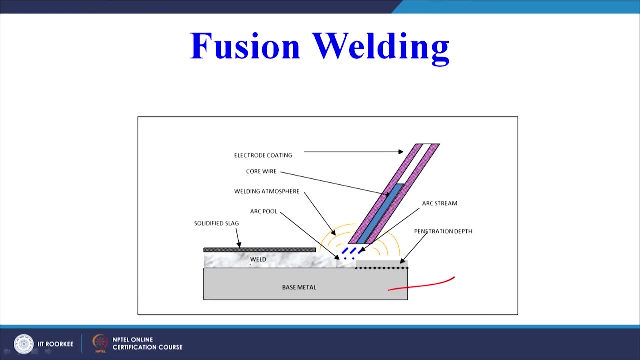 or by the application of pressure only, For example, forge welding or friction welding. so these are 2 broad classification of the welding processes. Now this is an example of the fusion welding process. we do it. this is the base metal, this is the weld that we are depositing. this is the electrode. it is a coated electrode. 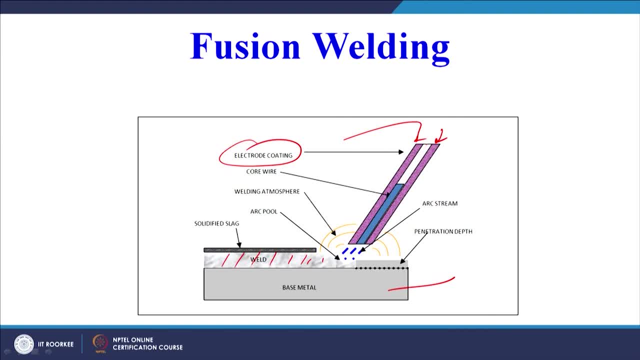 electrode coating is shown here. this is the coating and inside we have a electrode wire. So we have a core wire or the electrode wire, and this is the welding that is taking place here. So this is a simple example of electric arc welding process. 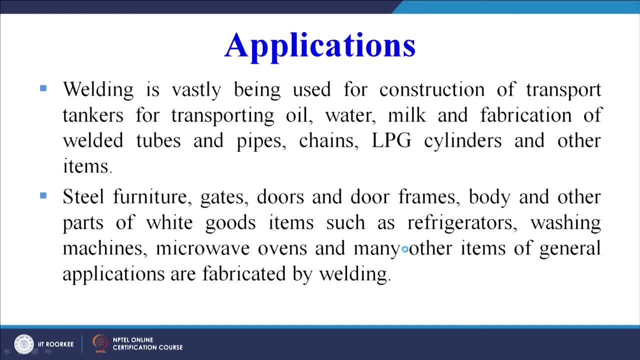 Now, what are the applications of welding? welding is vastly being used for construction of transport tankers for transporting oil, water, milk and fabrication of welded tubes and pipes, chains, LPG cylinders and other items. So you can see one of the application that we see in our day to day life. 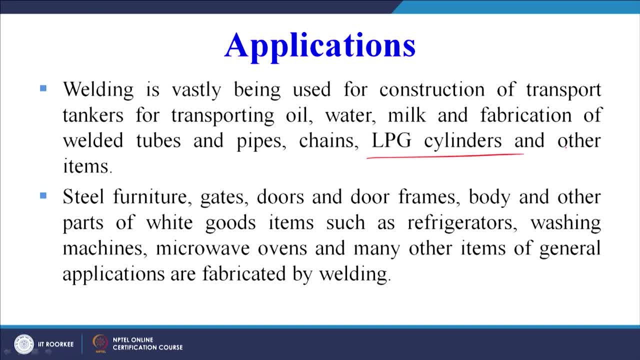 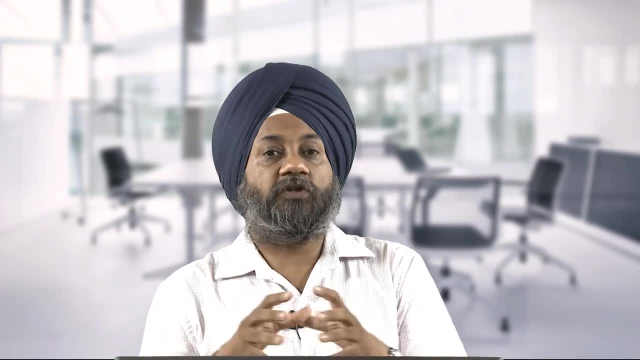 Steel furniture, gates, doors and door frames, body and other parts of white good items such as refrigerator, washing machines, microwave ovens and many other items of general applications are fabricated by welding. So I must summarize that welding is most important, Important, joining process which we see around us or for the products that we see around. 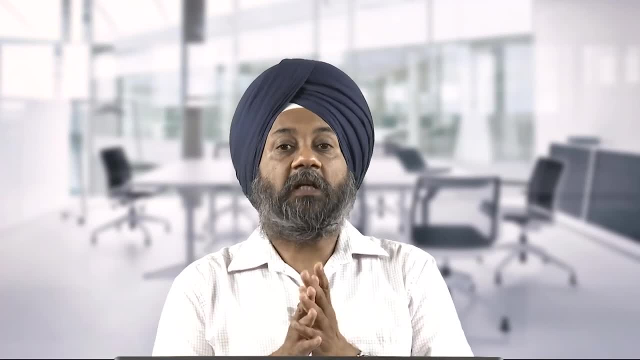 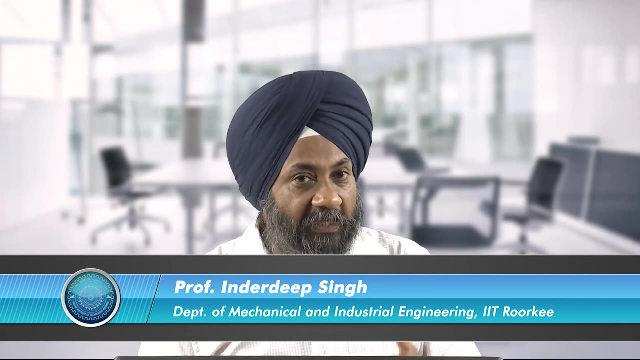 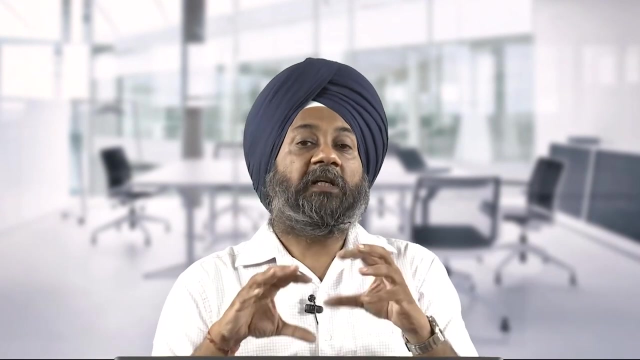 us. So with this we conclude the today's session. this was just an overview of the various joining processes, So now, subsequently, one by one, we will take a process each and try to see that what are the various guidelines that are established for designing of various parts which are to